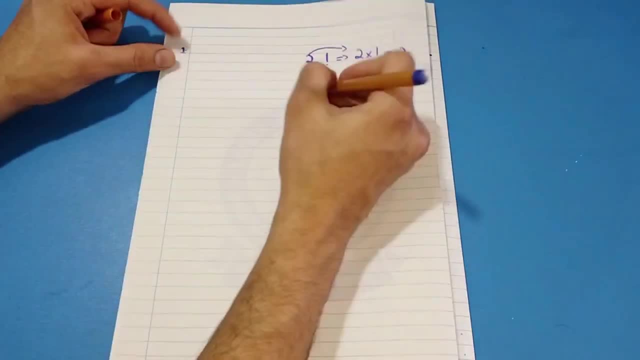 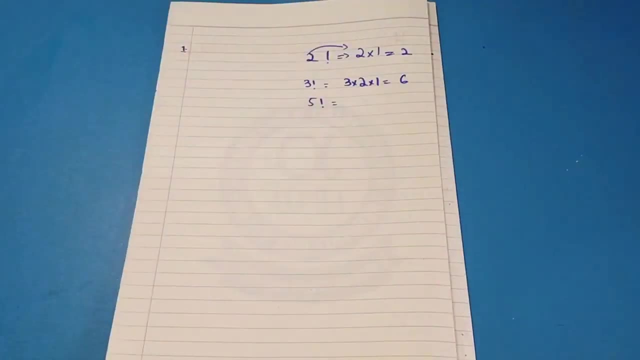 What is the value of 3 factorial 6? Okay, let's increase our talk further. For example, we have 5 factorial. So what does 5 factorial mean? From 5 to the previous number you have to multiply all the numbers. Means 5 multiplied by 4. 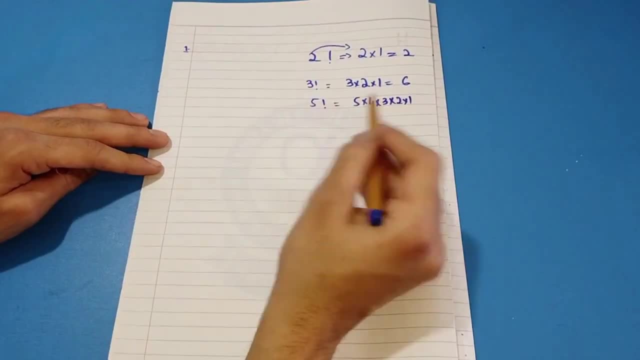 4 multiplied by 3, multiplied by 2, multiplied by 1, 5 multiplied by 4 is 20, 6 multiplied by 3 multiplied by 2, multiplied by 1, equal to 120. What is the answer of 5 factorial? My son? it is 120. 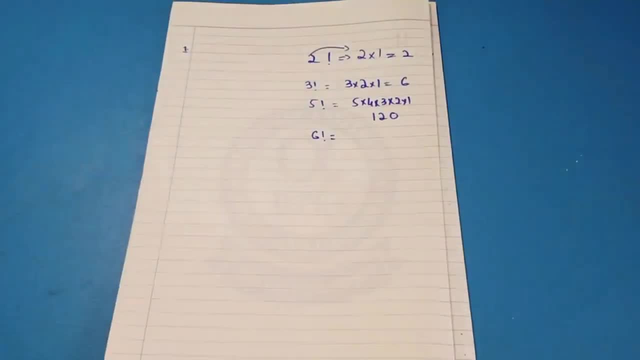 Same goes for here. What does 6 factorial mean? From 6 to 6, multiplied by 5, equal to 3. 3 multiplied by 2, multiplied by 1, equal to 1, Means you have to multiply all the numbers. What is the answer of 6 factorial? 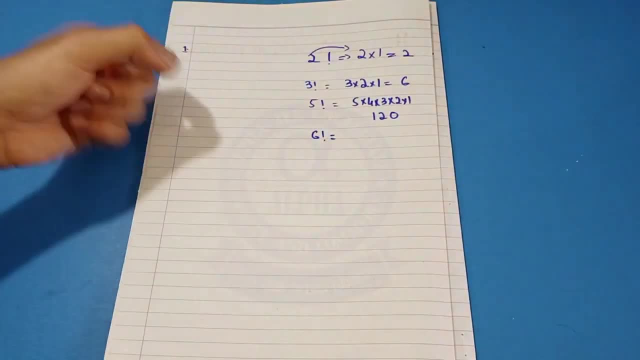 So you should know this thing before solving factorial: What is factorial, Although I know that many of you will be allowed to take the exam. But still you should know how to solve it without a calculator, Because in MCQ the data of the variables comes. Children get trapped in it. 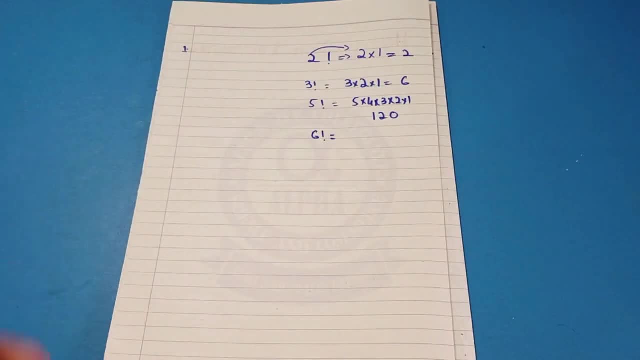 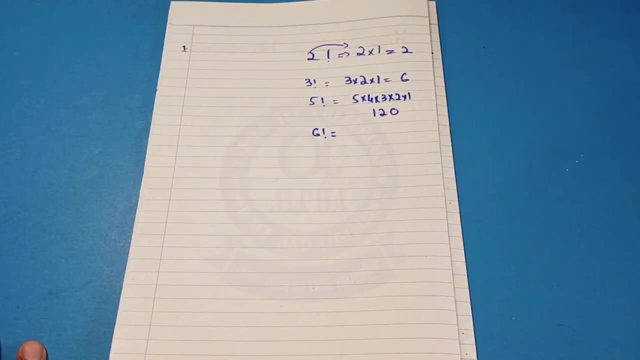 Or you don't look at the formula many times or don't look at the short tricks of the method. You are used to doing it on the calculator. When questions come in the aptitude exam, Then there is a problem. So see the concept in this way once. 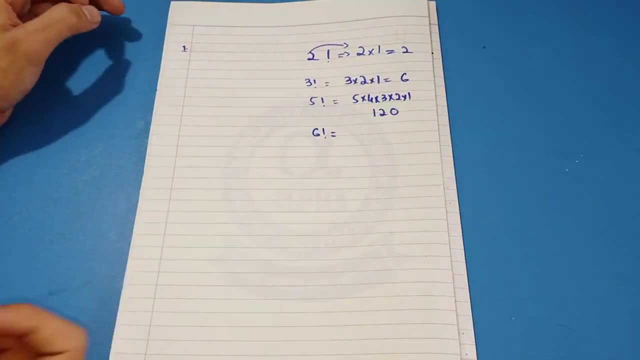 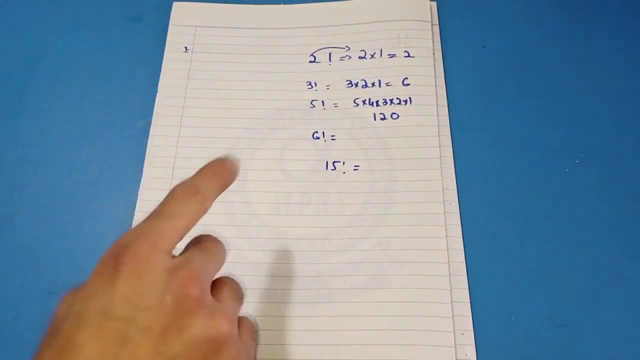 So my first concept is: Let me explain to you what factorial is. For example, when it is written 15 factorial, What does 15 factorial mean? How will the answer of 15 factorial come? 15 multiplied by 14, multiplied by 13, 12,, 11,, 10,, 9,, 8,, 7 till 1? 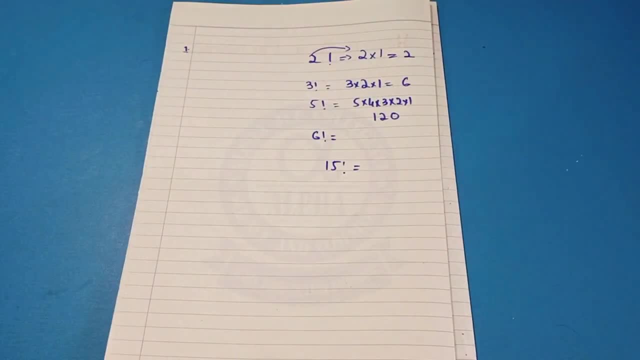 Let them multiply, Then the answer of 15 factorial will come. When it comes 80 factorial, It means that you will go back from 80 to 1. If you multiply all the numbers, then the answer will come. If I am doing all these things, Then there is no reason behind it. 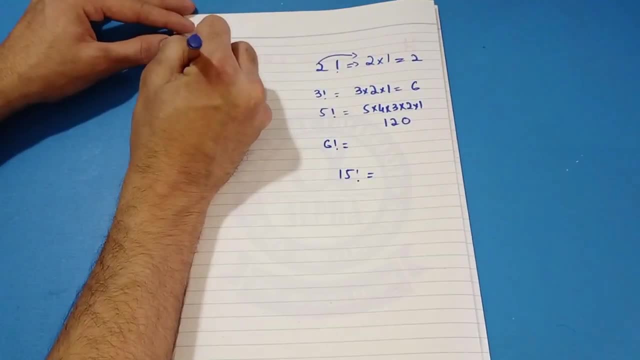 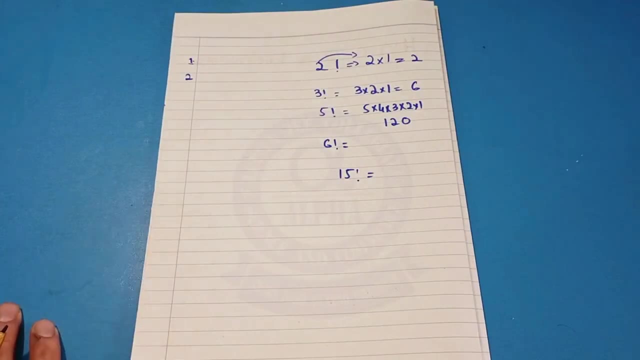 I also know that it can be taken out through the calculator. On the first number. On the second number, I will say one more thing to all the students. You should remember the answer of 6 to 7 factorials, So that you remember If you are preparing for the aptitude exam. 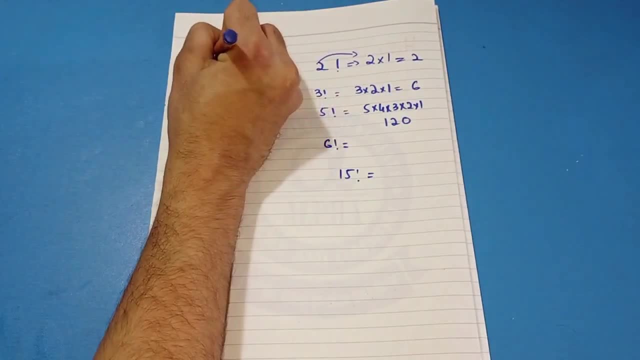 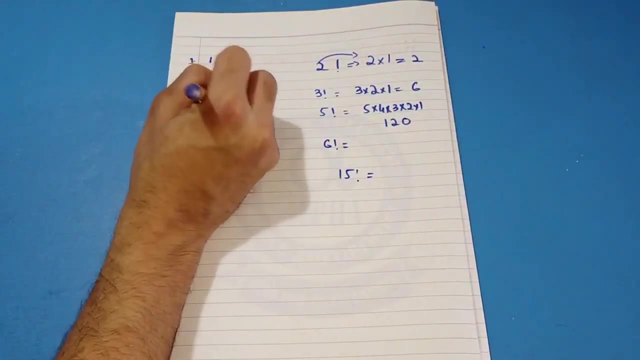 Then, kindly, kindly, you should remember the answer of 6 factorials. What is the answer of 1 factorial 1? What is the answer of 2 factorial 2? What is the answer of 3 factorial 6? What is the answer of 4 factorial? 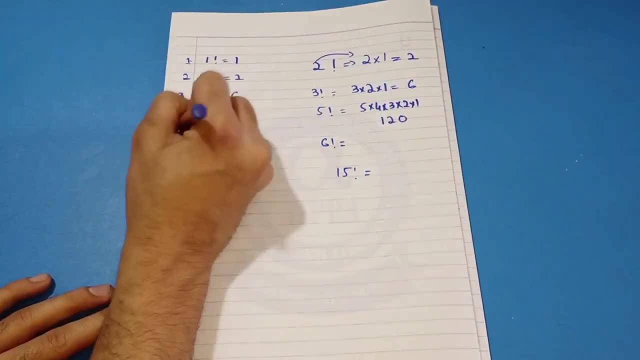 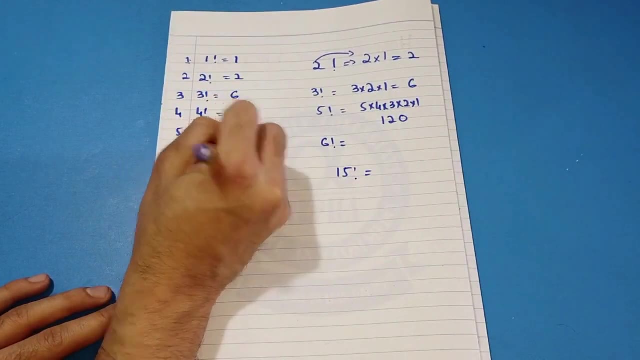 24. What is the answer of 4 factorial 24? And then on the fifth number, 5 factorial. what is the answer of 6 factorial? i guess answer of 6 factorial is 720. what is the answer of 6 factorial 720? 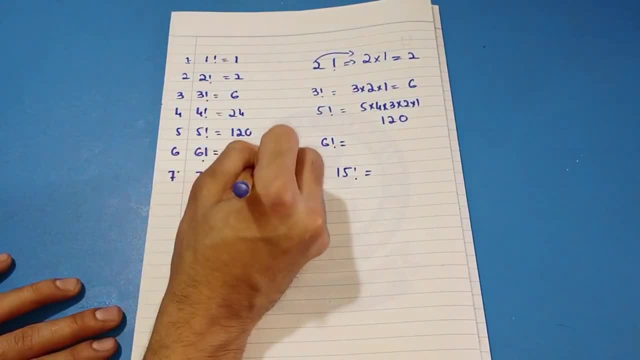 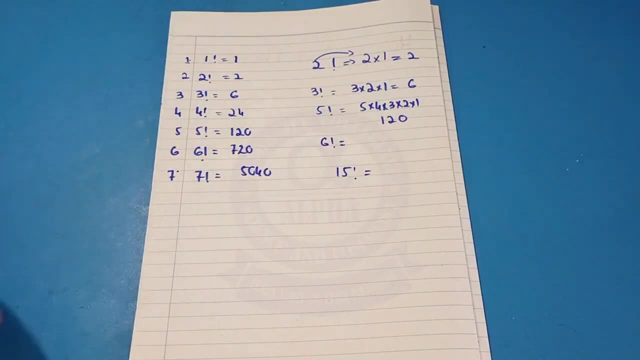 and then the answer of 7 factorial we are getting is 5040. if you want to improve your basic math, then kindly remember these 7 factorials. I know that you can't take them out with calculator, but still you should remember these factorials. 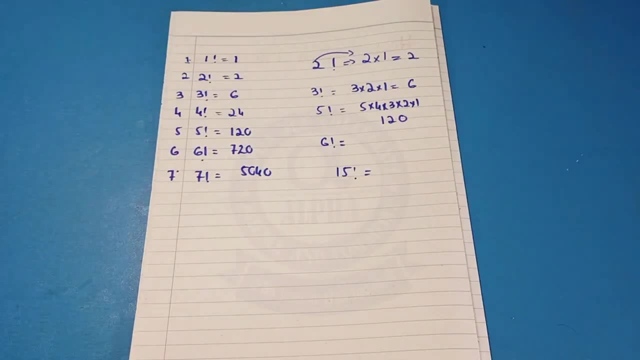 what is the answer of 1 factorial? what is the answer of 2 factorial, 3 factorial, 4,5,6,7? you should remember these basic 7 factorials. now let's come to the questions and see how we are getting the questions. 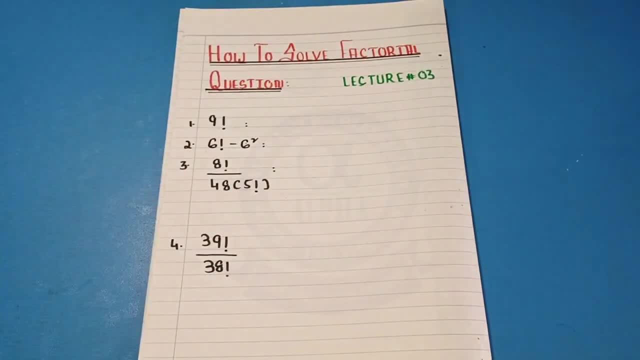 now my first question is: what is the answer of 9 factorial? now the student gets worried. if calculator is allowed in your aptitude exam or in your intermediate exam in first and intermediate exam, then you can easily take out 9 factorial. otherwise, if you are appearing on IBS side or NUS side, 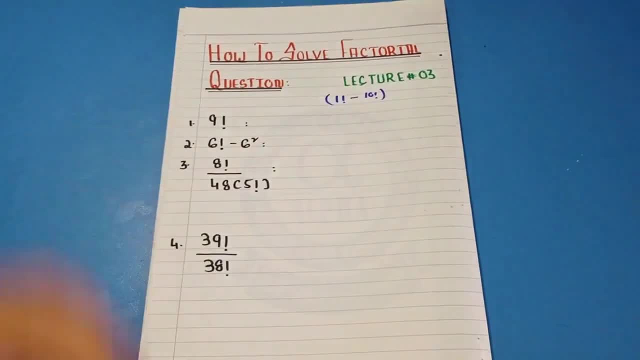 then kindly remember: from 1 factorial to 10 factorial. I will repeat it again: if you are appearing on NUS side or IBS side, then you should know the answer of 10 factorials. if you are preparing for intermediate and you are watching this lecture. 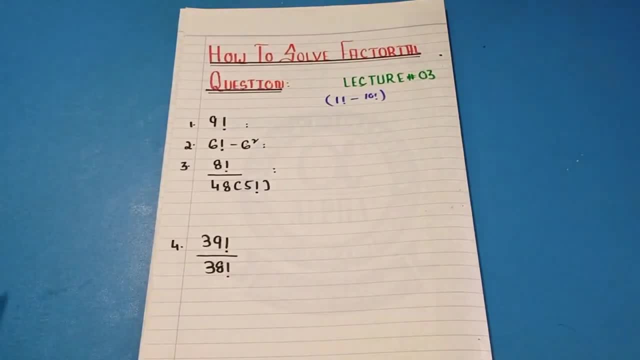 then you can take out 9 factorial from calculator. the answer of 9 factorial is 362,8,0. what is the answer of 9 factorial 362,8,0? I think this is the answer. 9 factorial is the answer if you are preparing for intermediate. 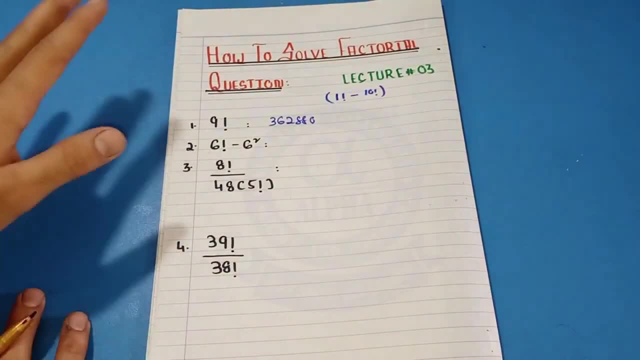 then you can do 9 factorial, but normally in intermediate there are no options of 9 factorial or 8 factorial in MCQs but in IBS side. if you are appearing on IBS side then kindly remember from 1 factorial to 10 factorial. 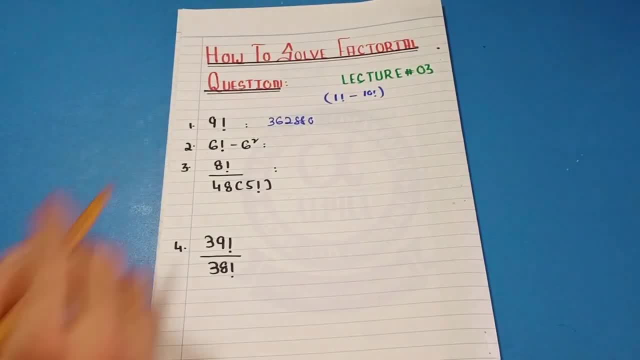 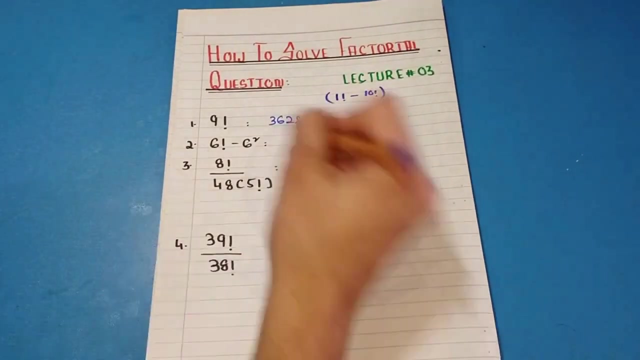 if you are preparing for intermediate, then kindly remember from 9 factorial to 8 factorial. the second question is how to solve factorial question. 6 factorial minus 6. square 6 factorial is 720. 6 factorial is 720 and minus sign. what is the square of 6? 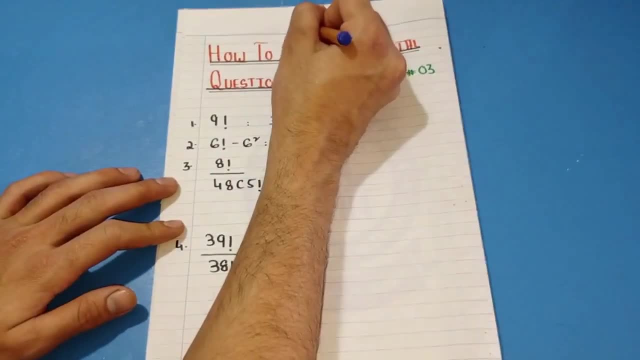 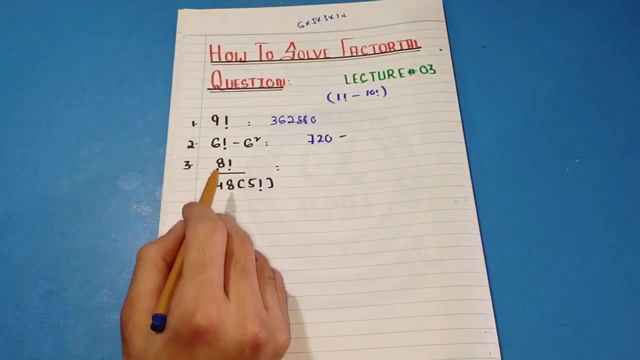 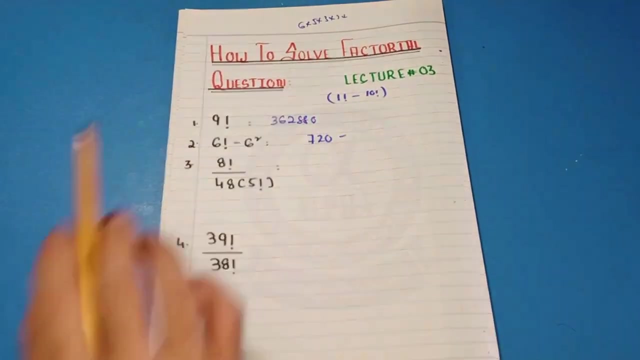 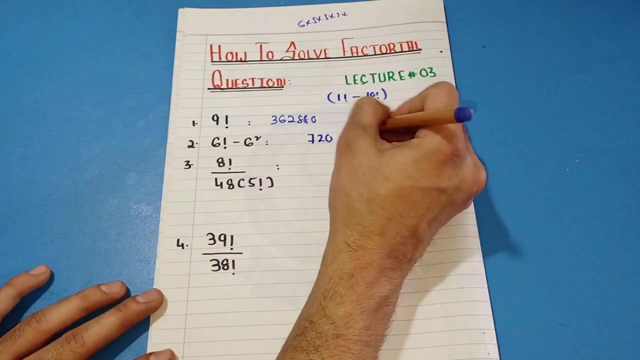 if you remember, then also you can do it when you are sitting at the exam doing like this. no, when you will remember, your time will matter. your time will matter. what is the answer of sixth factorial 720 minus the sign 6 square is 36. If you take out 36, then what will be left? 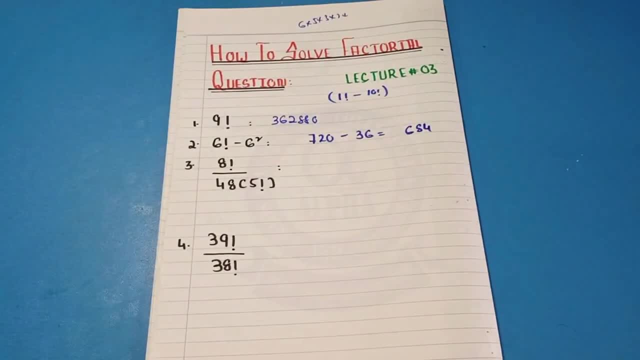 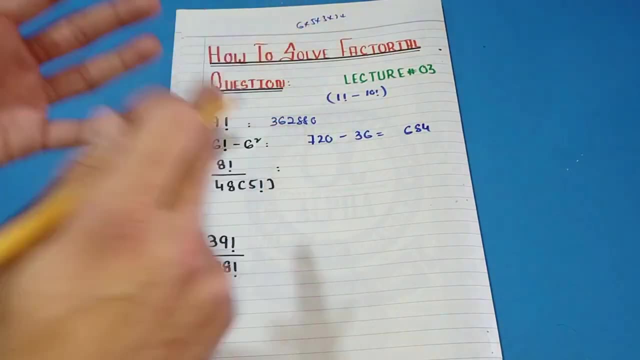 684. I guess What will be left? 684.. Such questions come in the paper. It is a basic question. If you remember 10 factorial in the beginning, then you can do 4.. If not, then you will keep it in your hands. 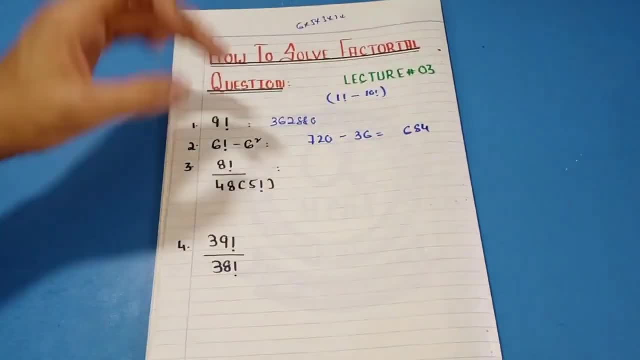 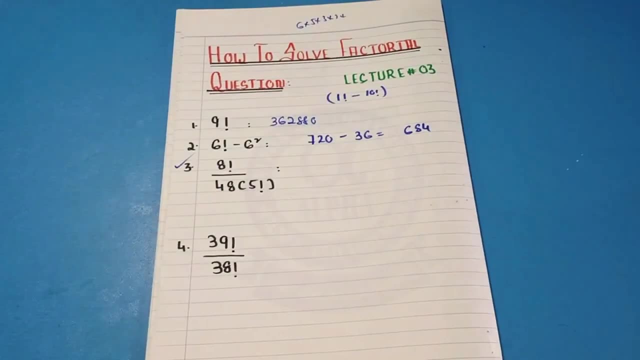 If it is 6 factorial, then you have to go from 6 to 1.. If you remember 10 in the beginning, then you will do such questions. Now look at question number 3.. This question comes a lot in MCQs. 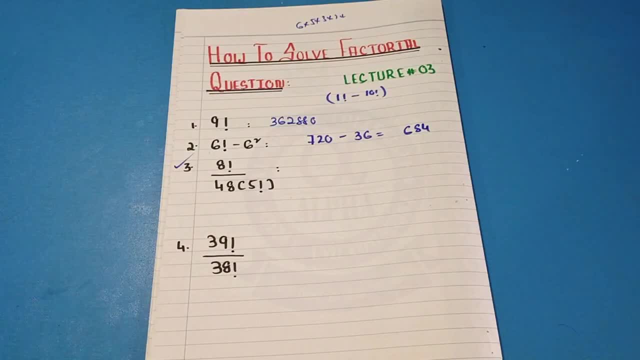 If you are giving a good paper or if you are giving a good aptitude exam of any university. Such questions come a lot in MCQs. What question are they asking you? 8 factorial divided by 48 into 5 factorial. It is a very good question. Now I will talk about logic. 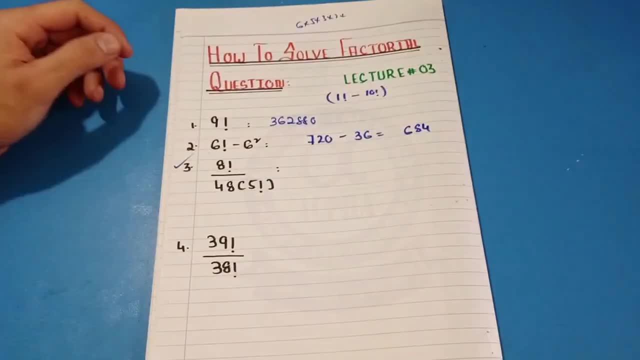 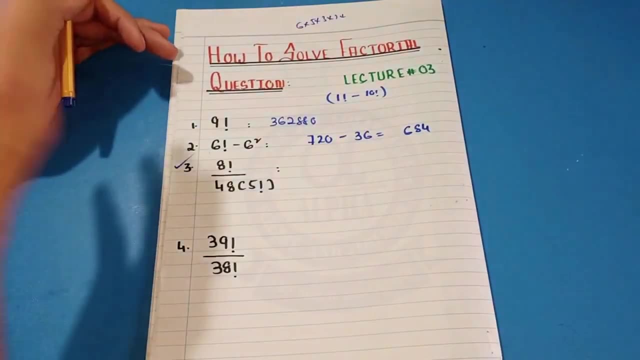 I have taught you once again in this video lecture what is factorial. What did I tell you? What is factorial? Factorial basically comes with any number or any element. You always go from that element or number to the back side Till where it has initials. 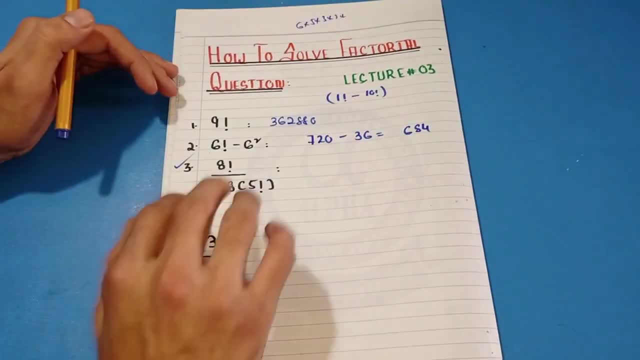 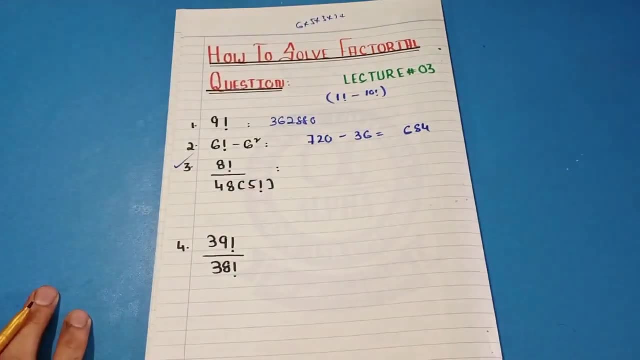 It is clear. Now we will see it in the form of variable. If you understand the number, then you will go to the variable. What is factorial? You go from that particular number or element to the back side, Till where it has initials or starting. 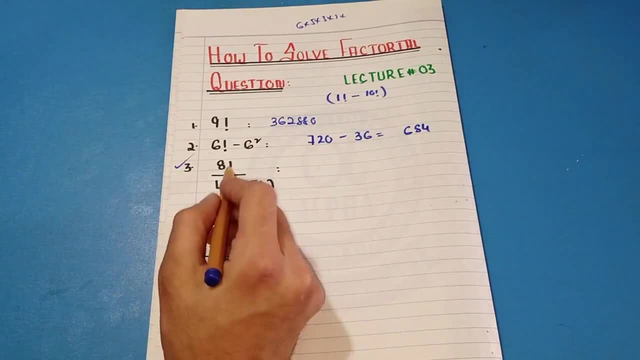 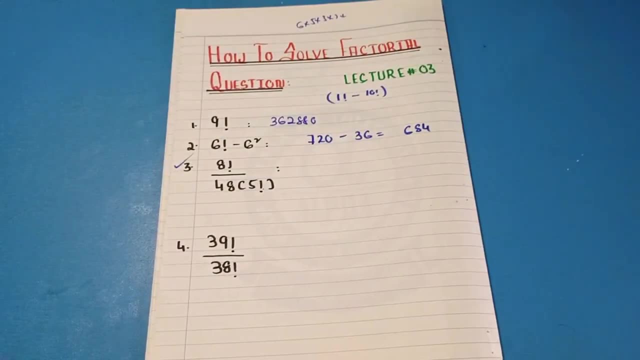 Are you able to understand what I am saying? I guess you are able to understand. Now see what is 8 factorial, What is 5 factorial below, Although I have taught you the value of 8 factorial And you also know the value of 5 factorial. 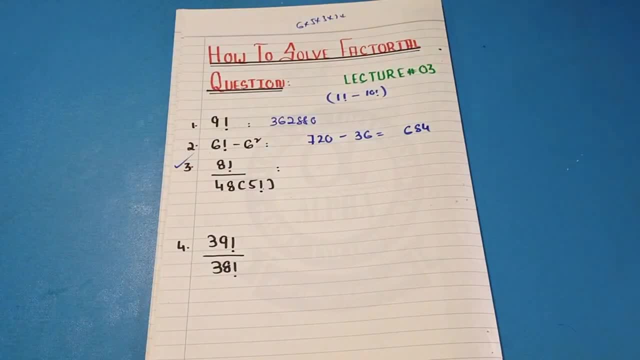 But for the sake of Allah, don't put the value of 8 factorial directly here. If you ever have 2 factorial, If you are dividing 1 factorial from another factorial, Then you always have to apply a short trick there. What is this short trick? Let me explain it to you. 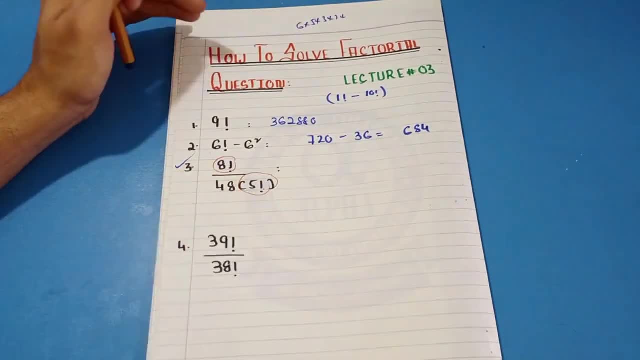 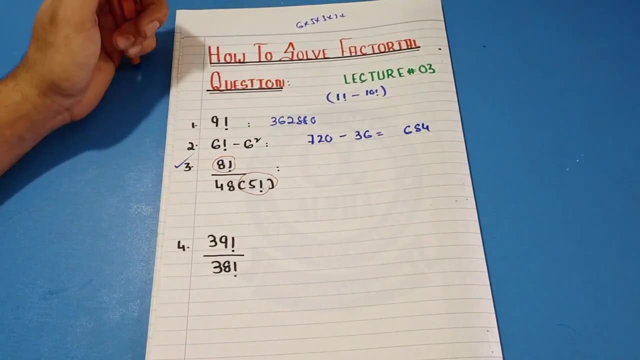 If you pay attention here, then what is happening? 1 factorial is above and 1 factorial is below. What did I say? If you are dividing 2 factorials from each other, Then you always have to apply a trick. What will be that trick? Whatever is above factorial. 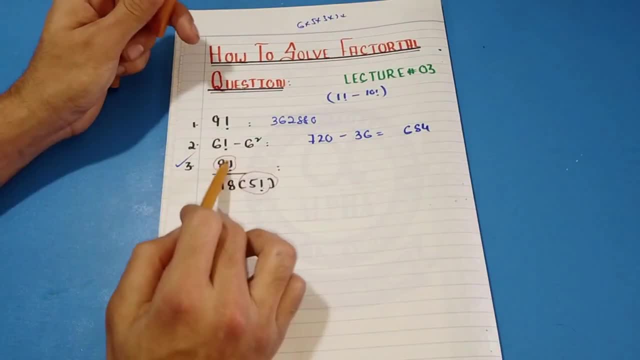 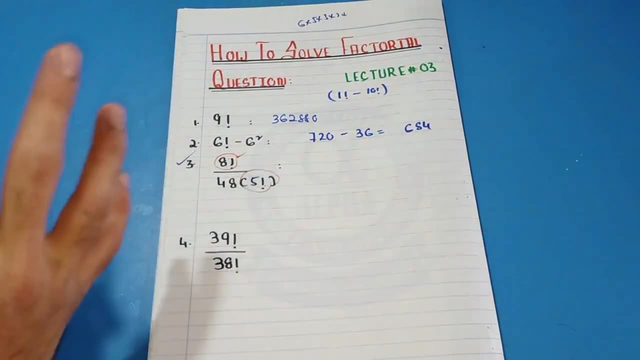 Or whatever is big factorial, in other words, Whatever is big factorial. If I have 2 factorials divided here- One is 8 factorial and one is 5 factorial, Which is bigger 8 factorial- So you will open the bigger factorial till there. 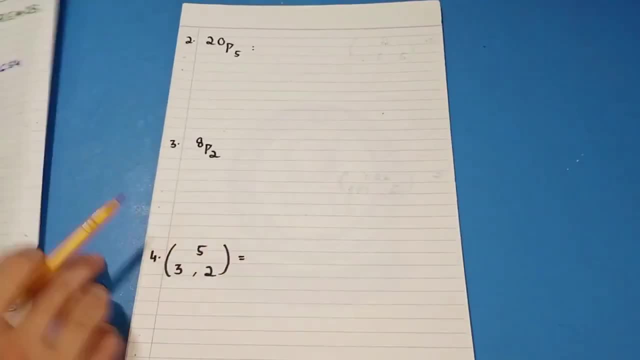 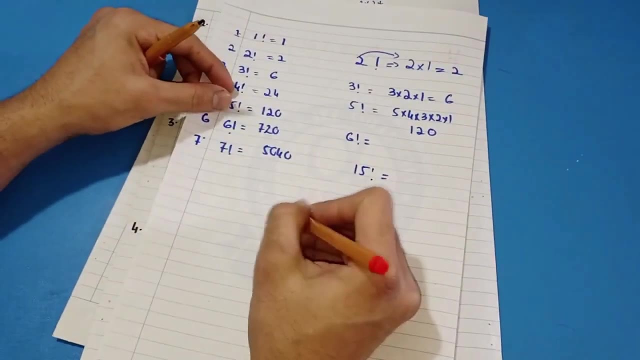 Till your next factorial is present. Sir, what are you saying? I don't understand. Let me explain it to you. For example, what did I say? If you are dividing 2 factorials, One is 5 factorial and the other is 2 factorial- 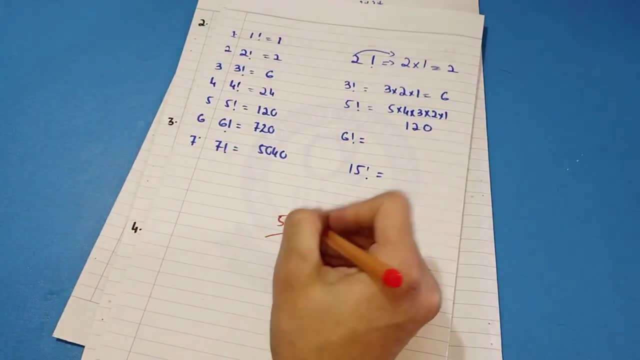 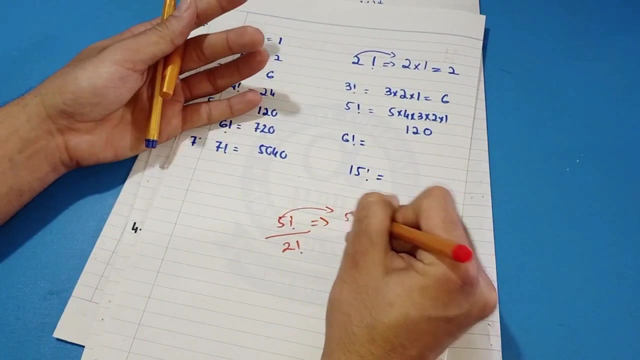 What is the meaning of my factorial? Factorial means that if it is coming with any element, Then this element will expand till there, Till 1.. So if I open it, then what will happen? 5 multiplied by 4, multiplied by 3, multiplied by 2, and then multiplied by 1.. 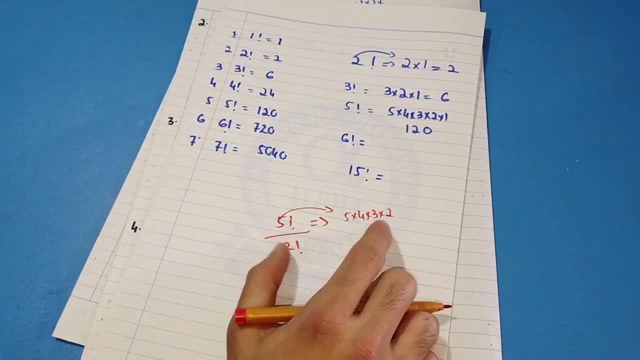 But if I stop at 2.. If I stop at 2. Because I can see that 2 factorial is coming below, And here I will put the sign of factorial, This means that I can cancel out the one above from the one below. 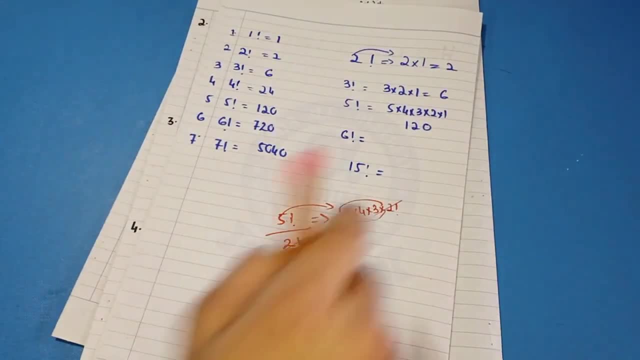 And this 5,, 4,, 3, which will come? The answer to divide both of them will come. I guess you didn't understand the thing. Let's see one more example. I said that if 2 factorials are being divided between each other, 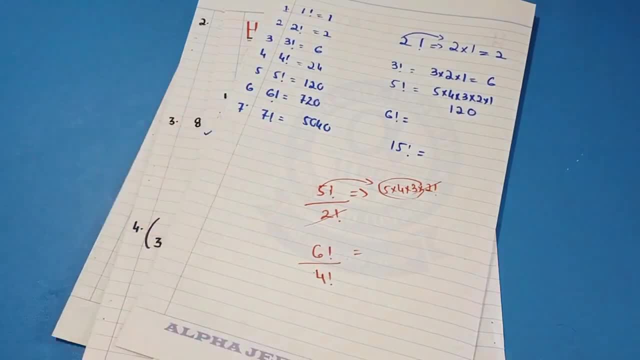 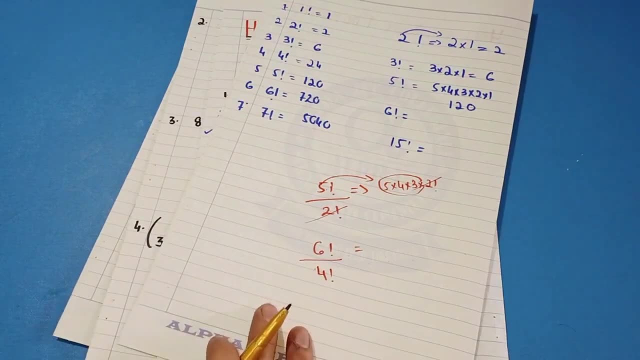 For example, 6 factorial divided by 4 factorial. I said that if 2 factorials are being divided between each other, Then there is a very good and beautiful way to solve them. There is a short trick that you can solve it without a calculator. 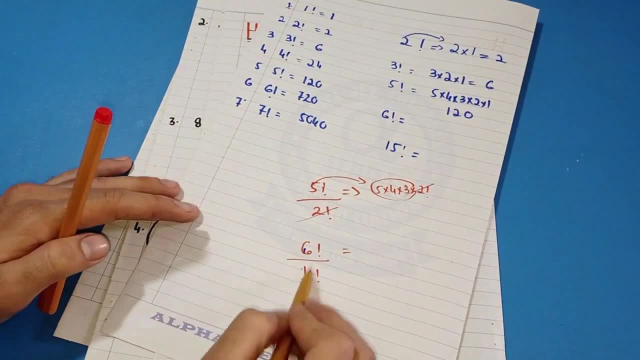 Look, I said that first consider the big factorial that you have. Which of these two is your big factorial? Is it 6 or 4?? Which is the big one? It is 6.. Now open 6 till there where your next factorial is present. 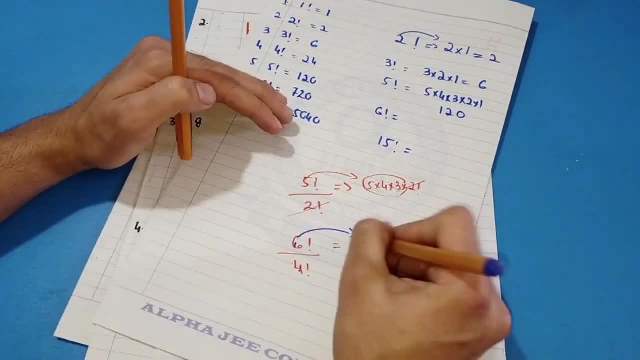 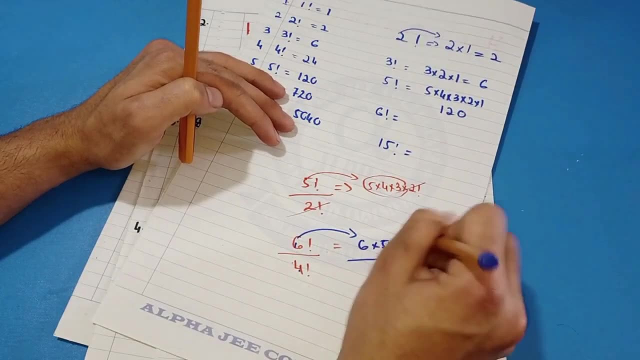 Now open 6 till 4.. And then put the sign of factorial on it. That means, what do I do with 6? 6 multiplied by 5, multiplied by 4. And I put the sign of factorial on 4. So that the factorial above can cancel out the one below. 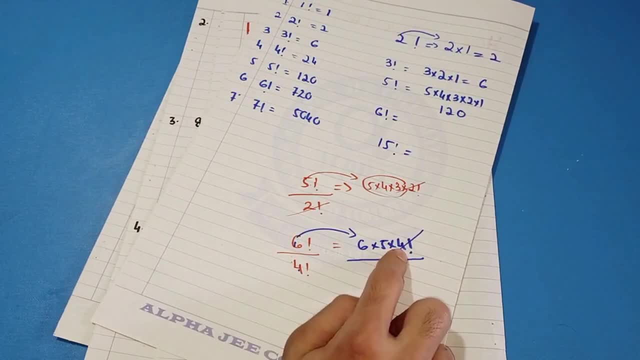 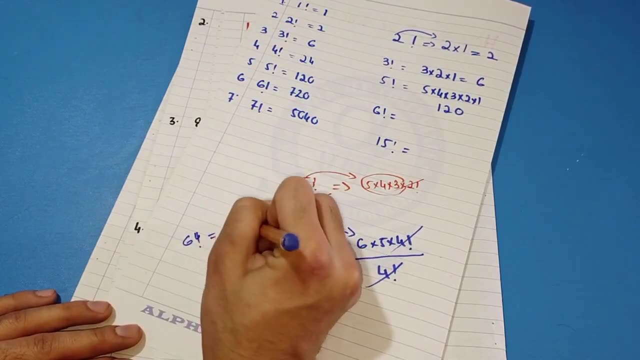 Sir, why am I putting the sign of factorial in your mind? How did I put the sign of factorial? So, my son, what is the original answer of 6 factorial? What will be the answer of 6 factorial? 6, multiplied by 5, multiplied by 4, multiplied by 3, multiplied by 2, multiplied by 1.. 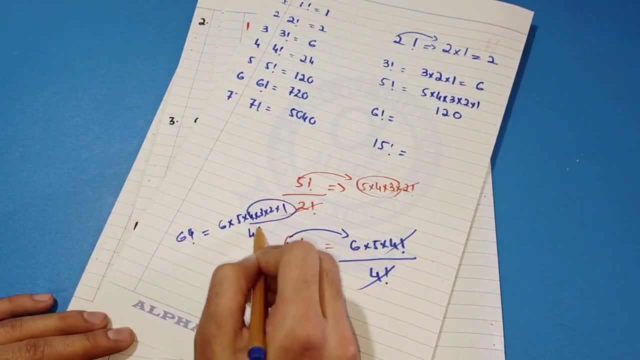 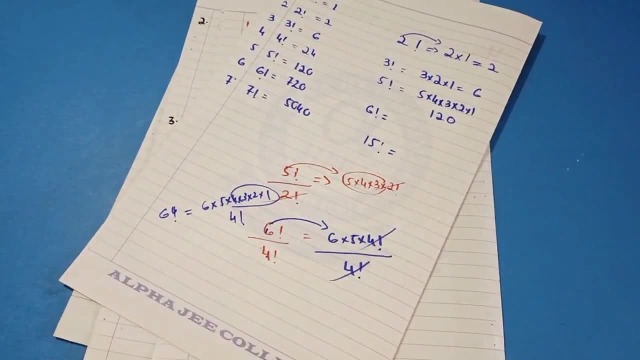 This will be the answer. If I put the sign of factorial above 4. So 4 factorial. If I put the sign of factorial after 4. Then it means that 4 can expand further. But I don't want to expand it further. 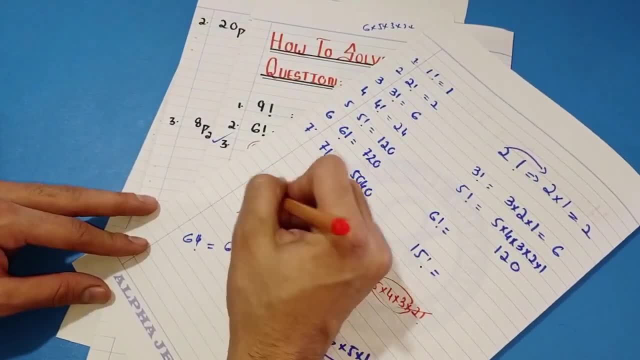 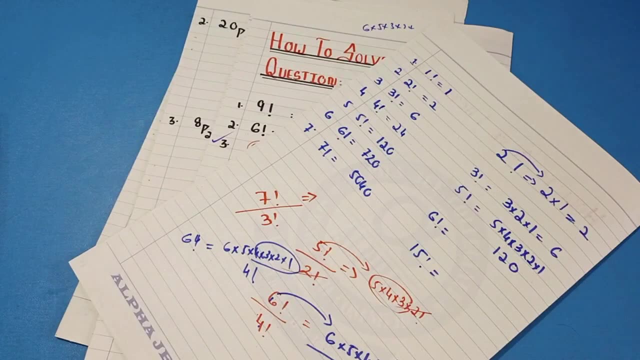 What is the purpose of saying this? Sometimes 2 factorials are being divided. That means, for example, 7 factorial divided by 3 factorial. You have to solve them And you should know how to solve without calculator. Calculator doesn't allow you. 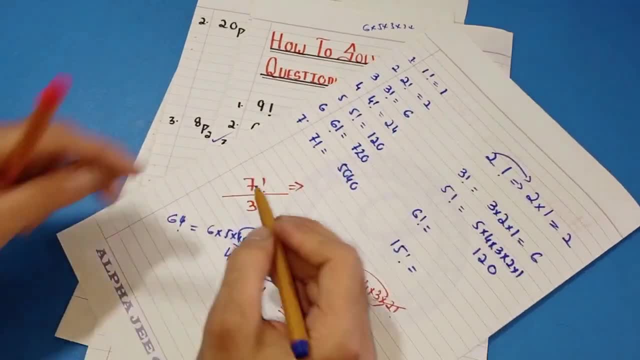 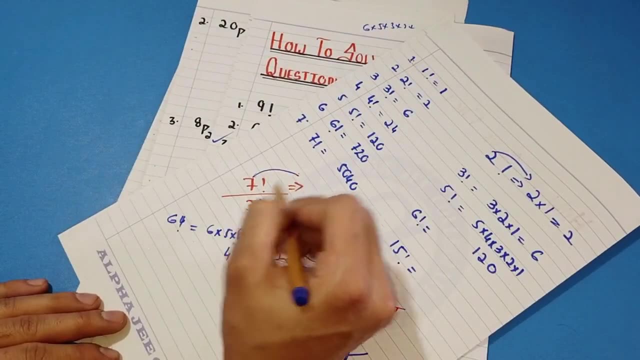 You should know how to solve. How will we solve? Let's understand this thing. 2: factorials are being divided. See the biggest factorial. What is coming? 7 factorial is coming. Expand 7 to the point where your second factorial is present. 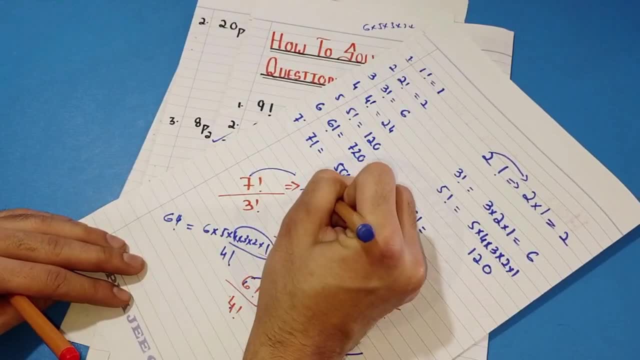 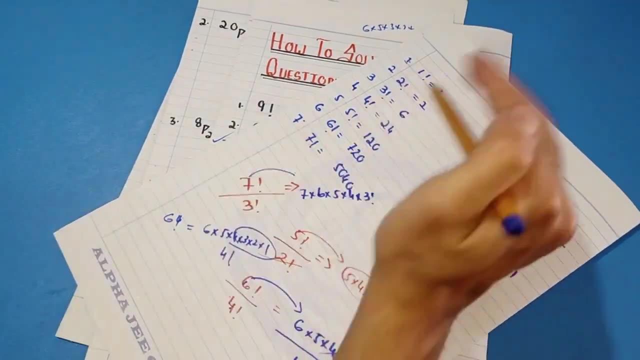 Where is the second? It is 3.. So what can I write it? 7 multiplied by 6, multiplied by 5, multiplied by 4, multiplied by 3, factorial. Here I stopped it at 3.. I don't want to expand it further. 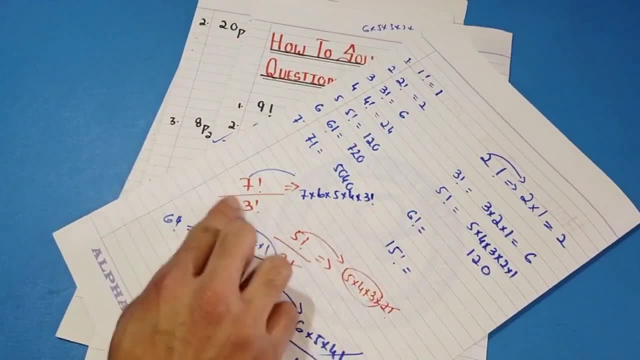 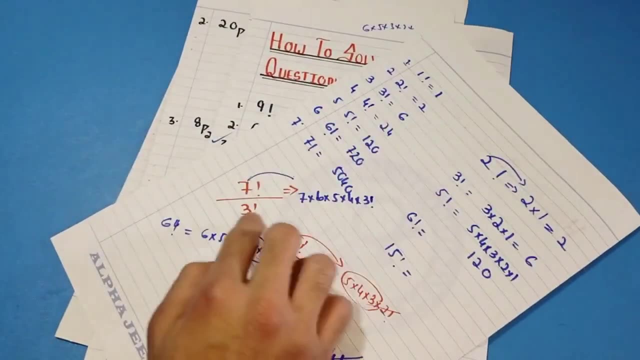 And I put the sign of factorial here. Why did I put this sign? Because 7 factorial, Because it expands till 1.. Because 7 factorial has to expand till 7.. But, But because 3 factorial is coming below me. 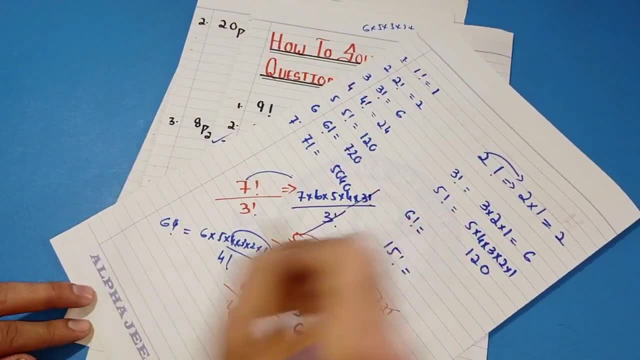 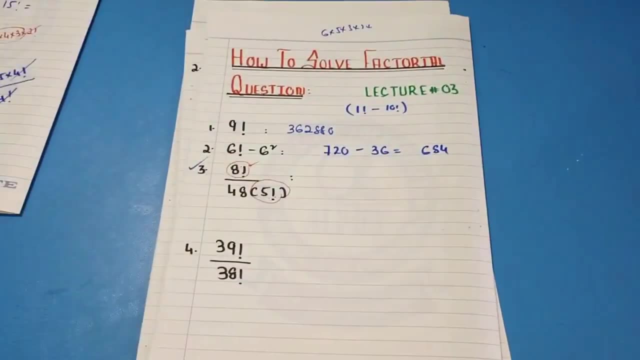 I want to cancel it out So that my solution becomes easy. That's why we will open the sign of factorial as much as the second factorial is coming. I guess I would have been able to clear my point. Now let's come back to this question. 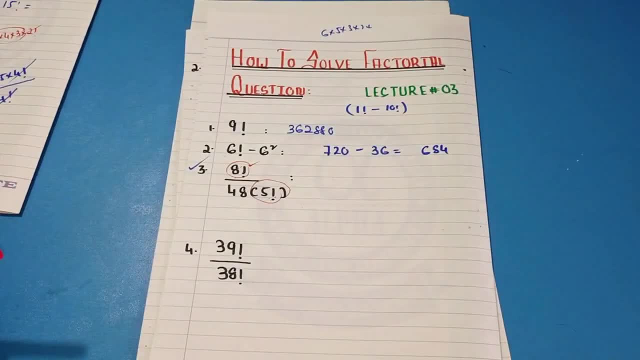 What is this? 8 factorial divided by 48 into 5 factorial. That means I have to solve this question Now for the first time. a child will see this. Sir, this is a very difficult question. The calculator is not allowed. 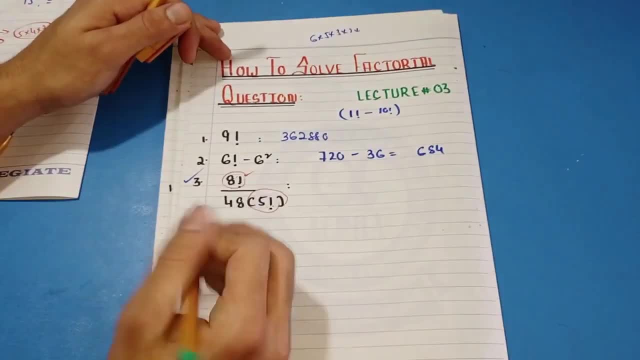 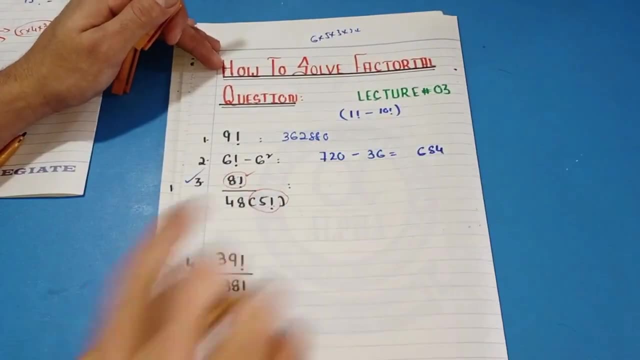 What will we do? My son, you should know how to open it. How will we open it? Look at the big factorial sign between these two. What is big? It is 8.. That means we will open 8 factorial Till where? 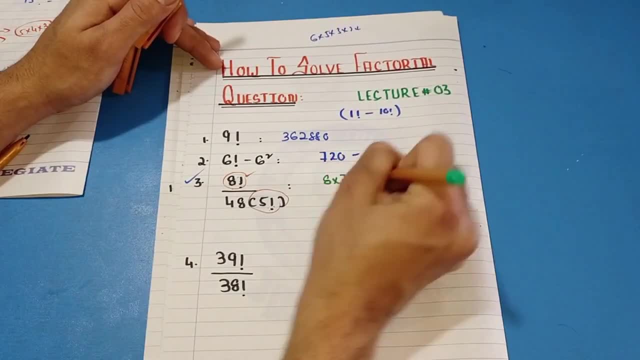 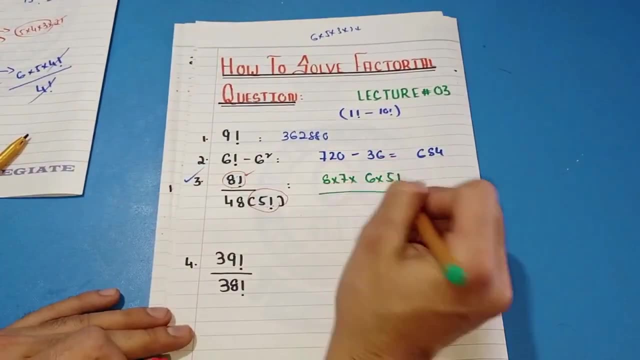 Till the bottom 5.. So what will become? It will become 8 multiplied by 7, multiplied by 6, multiplied by 5.. And we will stop it by going to 5. Because we will put the sign of factorial here, So that the factorial below- which will be 5, will cancel it out. 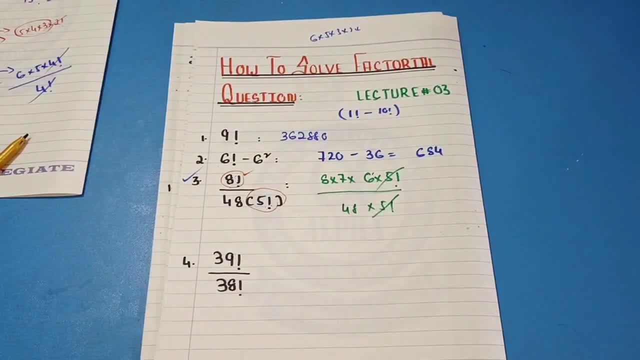 What happened, my son? This is our cancellation, And then we can solve the numeric number easily. And we will solve it very easily, Because what was the question? 8 factorial divided by 48 into 5 factorial. So what trick did we solve? 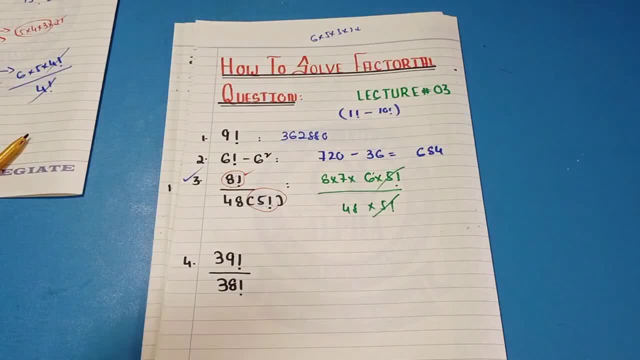 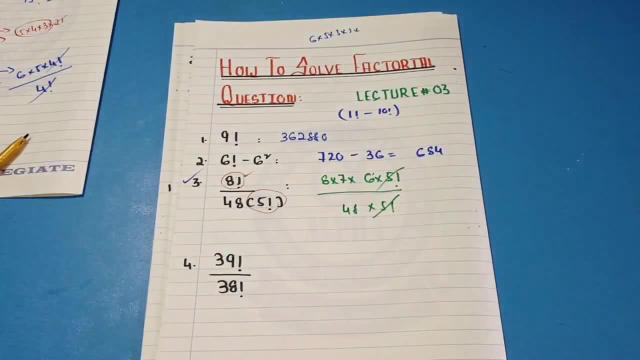 We will expand the upper factorial or the big factorial till where your second factorial is coming, Because here the big factorial was 8 factorial and the small one was 5. So we expanded the 8 factorial to 5. That means we opened it. 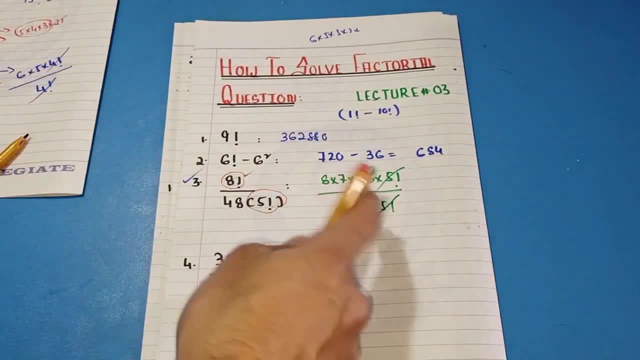 And then we cancelled 5 factorial from 5 factorial. So what numbers will come? 8 multiplied by 7, multiplied by 6, multiplied by 48.. If you think the numbers which are coming, 8 multiplied by 6, multiplied by 48.. 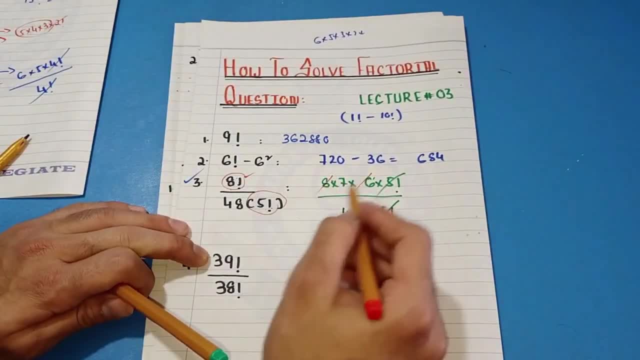 So we will cancel out the upper 8 and 6 multiplied by 48. Because 8 multiplied by 6 multiplied by 48. And 48 multiplied by 48. Obviously it will be 1.. So what happened here? Only 7 was left. 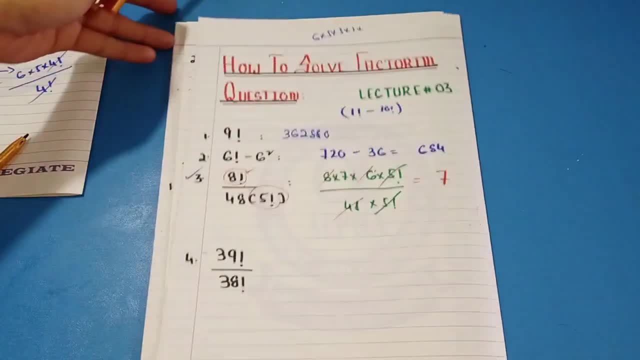 So the answer of this particular term will be 7.. My son, these are the tricks of quick maths. You should definitely know this If I teach this in chapter number 7. And in a different lecture So that you don't get burdened. 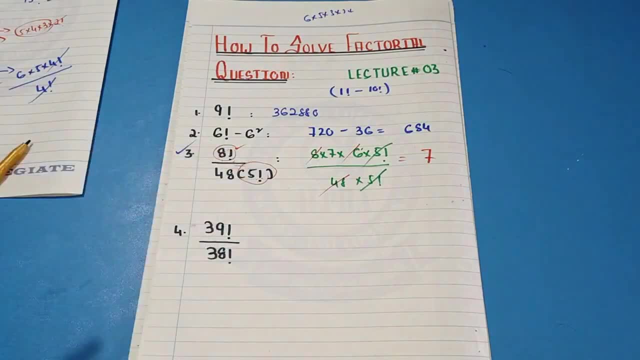 The main reason is that these are major things. If you understand these small things, Then we will go to the difficult questions. You will understand that easily. I told you in the starting, before starting, chapter number 7.. My son, chapter number 7, is very basic maths. 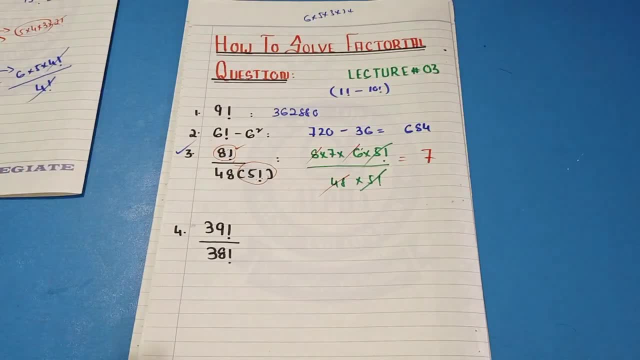 And this is the chapter which is extremely important- On the intermediate side also, And then on the aptitude side also. Whether you copy set series or net series, These questions are always coming to us. Okay, So I guess we understood this concept. 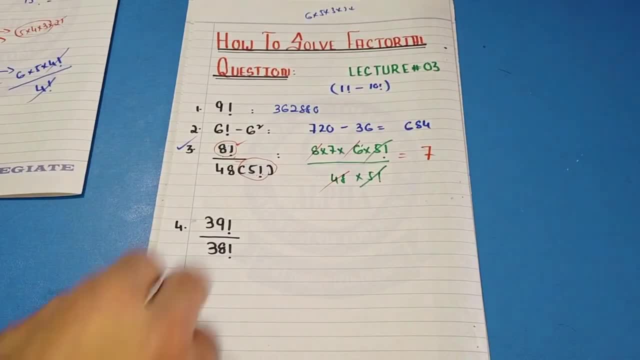 Now another concept has come. What concept is coming? That two factorials are being divided between each other And it is said to you to get its value Now, for the first time, a child will be scared to see this, Sir, such a difficult question. 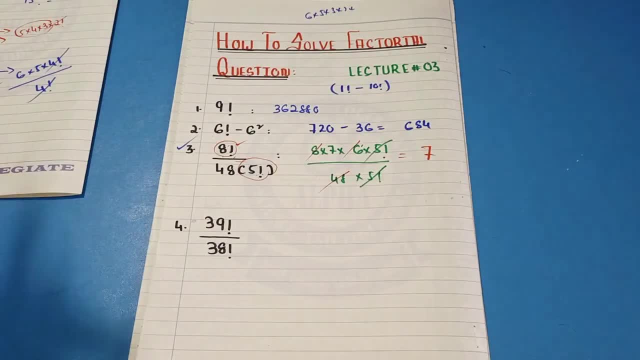 Oh God's people. it is an extremely easy question, Sir. how easy is it? Let's see now, son, What did I say to you? That two factorials are being divided between each other And you have to get its value. 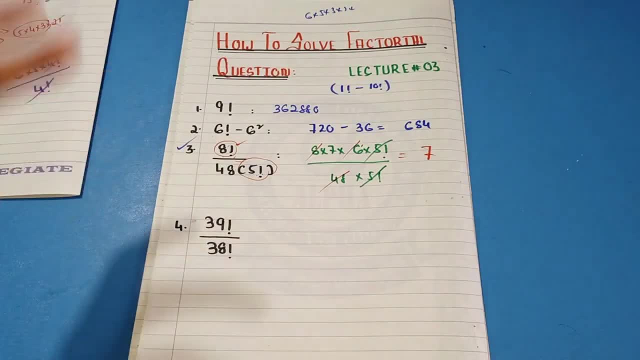 So, my son, you should also come without a calculator. If you do it with a calculator, then what is the matter of Suramkhan? Every child can take out a calculator from it. Take it out without a calculator, So that tomorrow it will be easy for you in your exams. 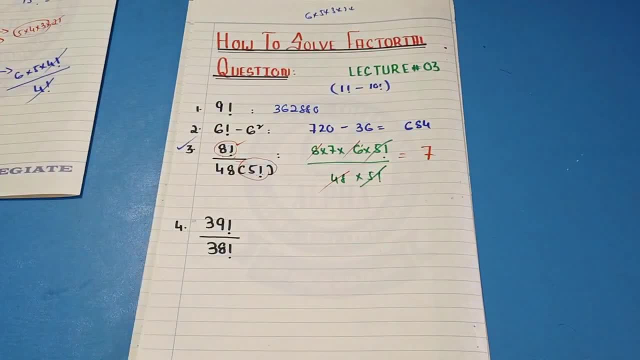 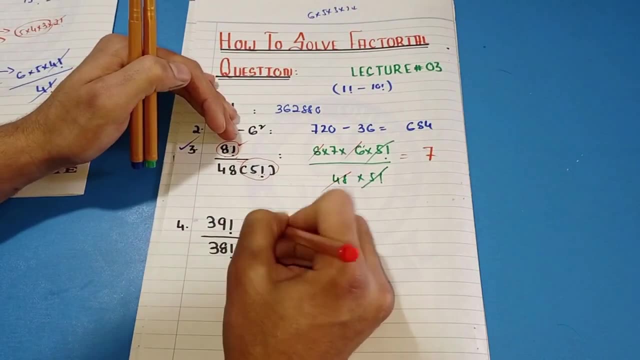 What is it saying? Thirty-nine factorials divided by thirty-eight factorials. What you have to do first is to check which is the biggest factorial among them. Of course it is thirty-nine factorials. It is a big factorial, Okay. 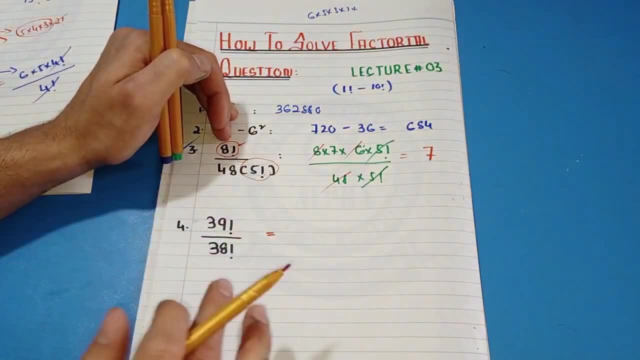 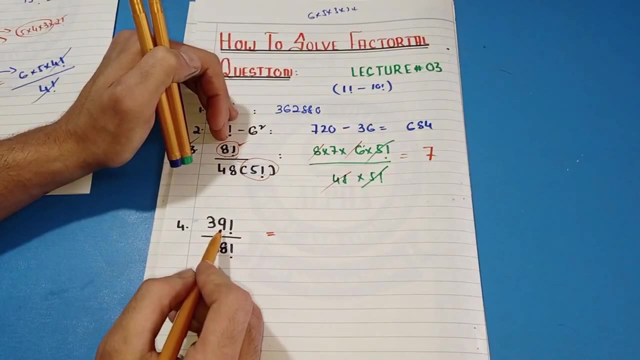 And what is thirty-eight factorial below? So you will expand your big factorials to the extent that you get another factorial, Because only then our answer will be a proper number. So what is coming here is thirty-nine factorials. What is coming below is thirty-eight factorials. 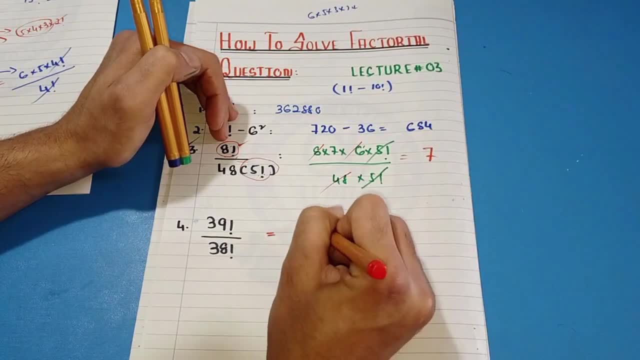 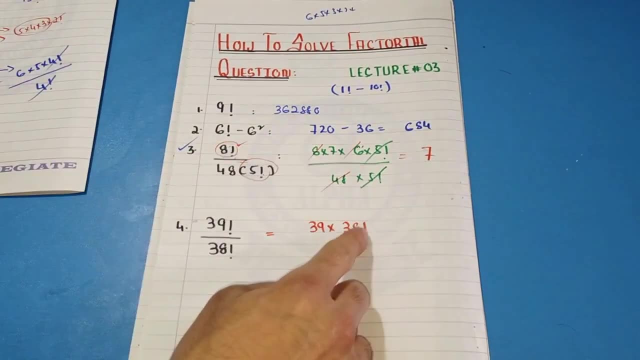 So what do I do? I expand thirty-nine factorials. So what will become? thirty-nine multiplied by thirty-eight, And I stop at thirty-eight. Now, thirty-eight factorials, I stop at thirty-eight. If I solve it further, then obviously it will go to one. 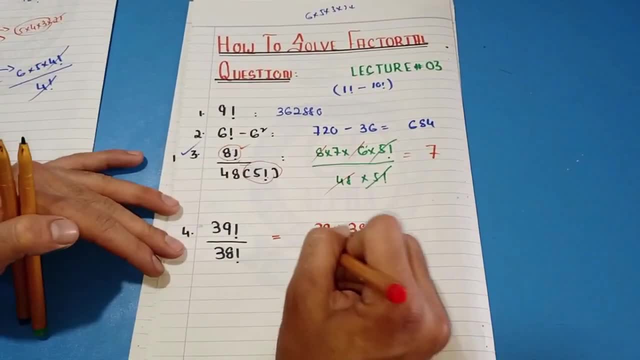 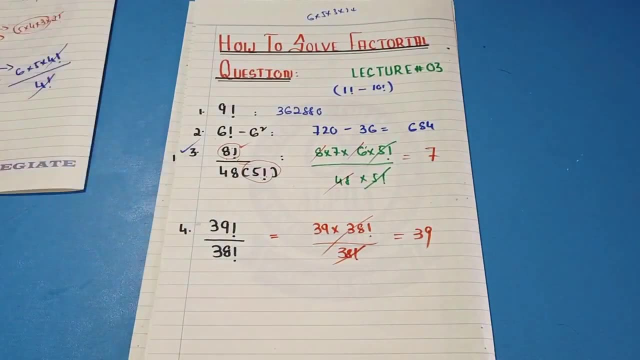 But because I stop it here so that God can cancel out the thirty-eight factorials below. then, simply, I will get the answer thirty-nine. In this way we are solving the question of factorials on these short tricks. If you understand the question of factorials, of numeric, then you will understand the question of variables as well. 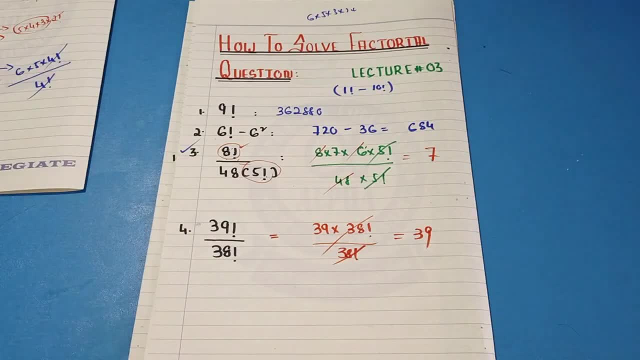 And the variable ones come more in the paper. Is my son clear? So what have we studied till now? I will quickly review you. What are factorials, How to solve factorials? I will tell you a simple thing: If you are having problem with someone, then I am ready to repeat again. 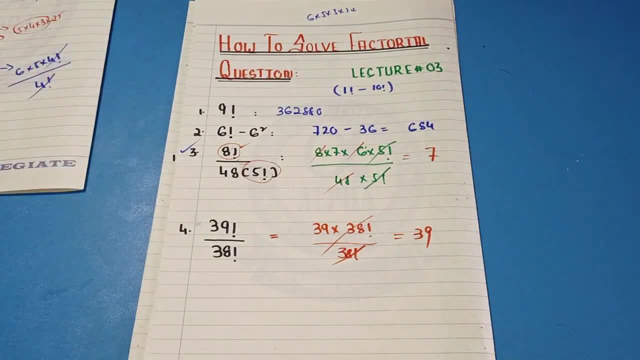 In any case, I am coming in, two factorials divide and you want to solve them. So, my son, it is a very easy way to solve them. Sir, what is that easy way? That easy way is that you will always check that brother. 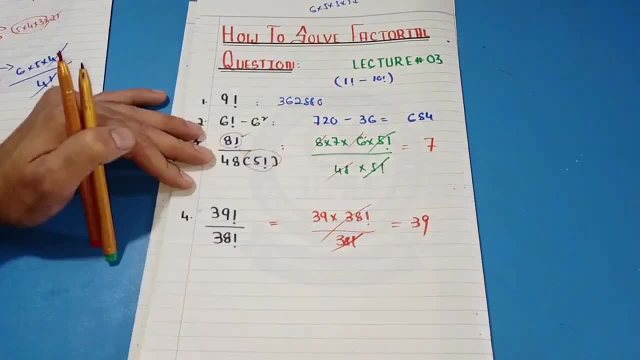 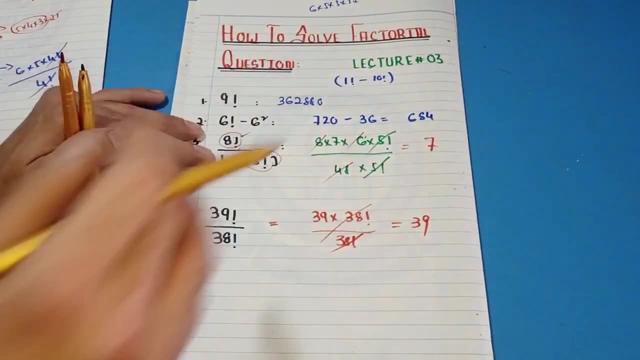 your upper factorial or your big factorial. Leave the upper one, the big one, Which is that and which is the one below, Meaning what is the small factorial- And then you will expand your big factorial so much that you have to cancel out the other factorial and get a simple number. 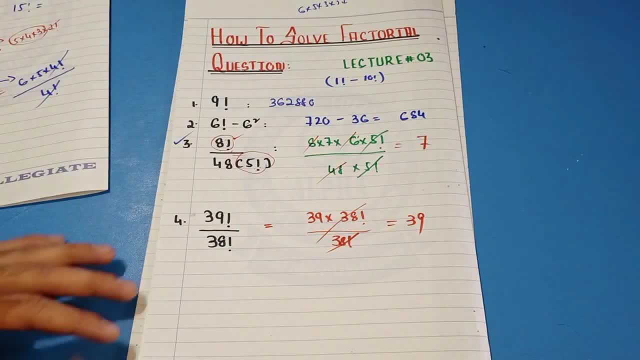 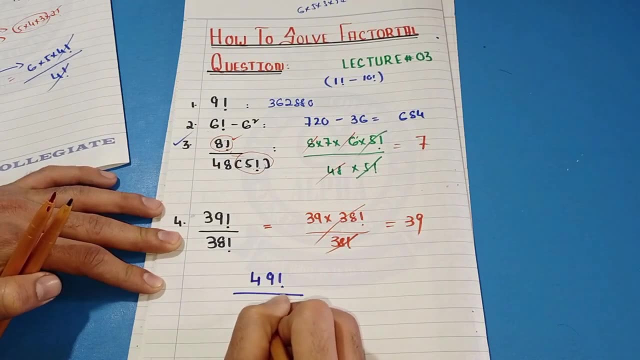 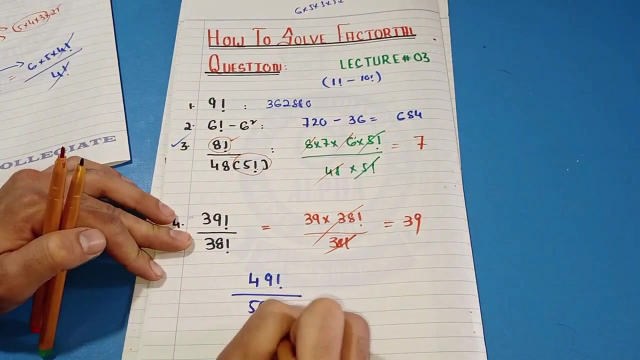 Sir, can you give any other example of this, My son? I will give you one more example of this. If you want to clear your words, then see one more example: 49 factorial divided by. What should I take here? I will take here 50, 50 factorial. 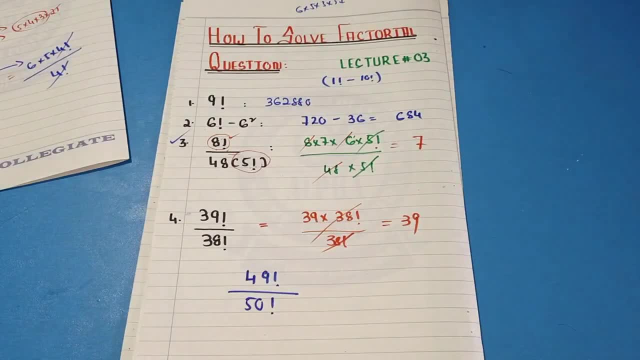 Now see. now see what I have: 49 factorial divided by 50 factorial. Sir, this is a very difficult question. You don't have to do it on the calculator. You should be able to do it by hand. How will you solve it? I just said one thing. 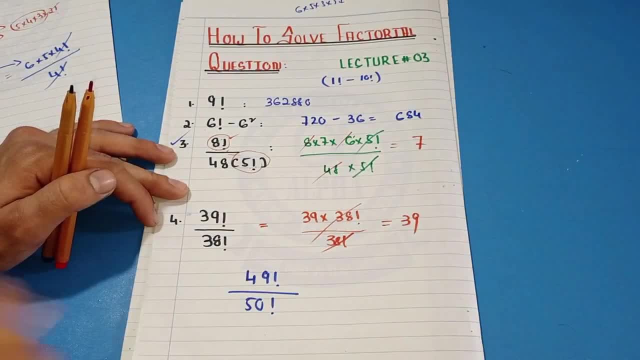 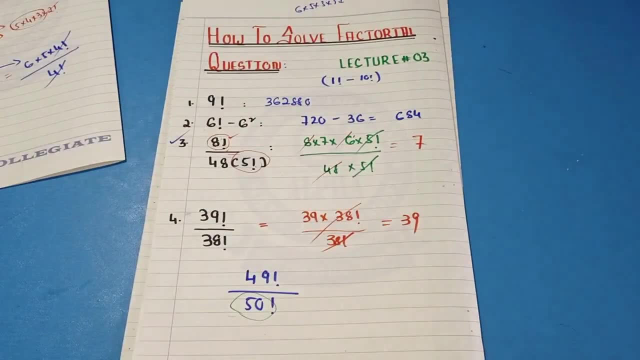 I said, the first thing you have to do is you have to see which is your big factorial. Which is the big factorial here? It is 50 factorial. The property of factorial is that it expands to 1.. That is, it will go from 50 to 1 by multiplying. 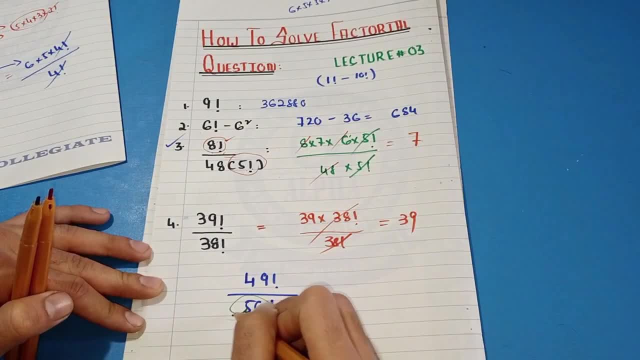 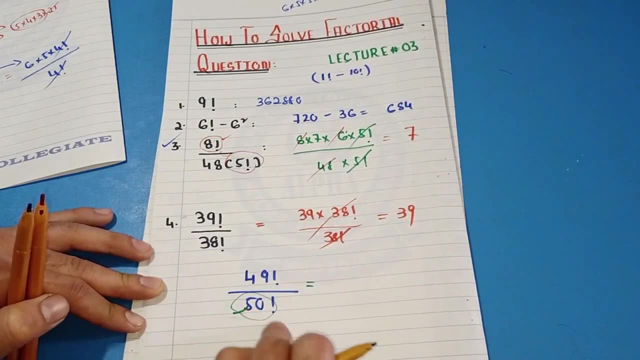 But you have to check that which is the big factorial and which is the small factorial. I clearly saw which is my big factorial, which is 50 factorial and which is 49. That is, I have to divide my 50 factorial and expand it and stop it. 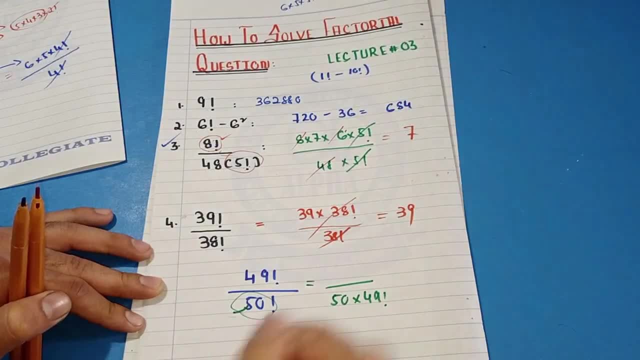 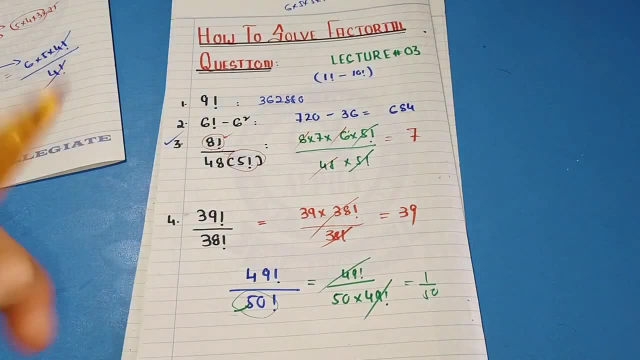 So what will happen? I will stop 50 multiplied by 49 factorial here And above 49 factorial as it is. So 49 factorial is cancelled out. So the answer will be 1 divided by 50.. Is it clear, my son? 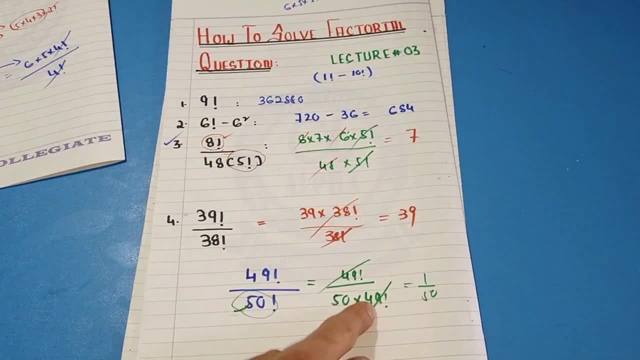 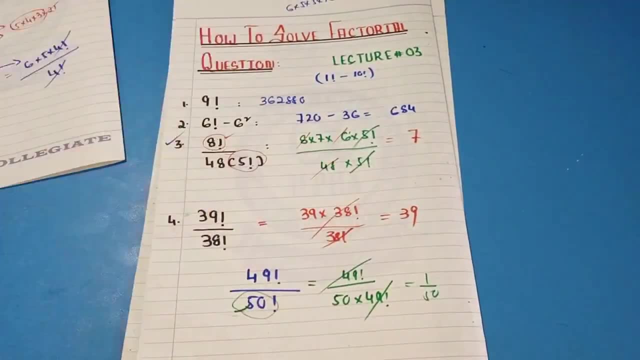 I guess now it will be clear. after all the people: Okay, we stop here because so that we can cancel out the other factorial's sign. I don't think there should be any issue in this. We expand factorial and stop it so that we can cancel out our other factorial part. 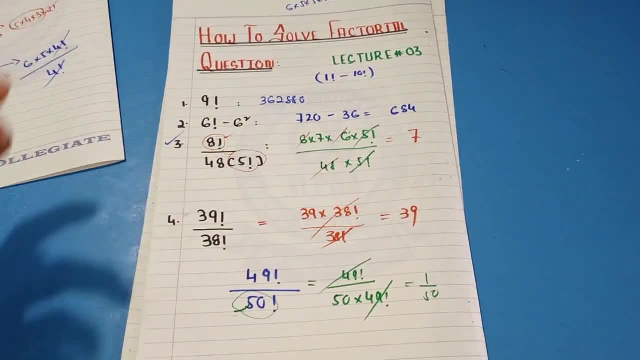 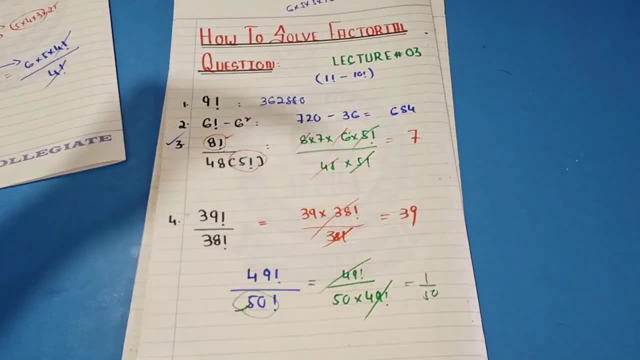 So what have we read till now? son That, how do you solve basic factorials? And then, if there will be the sign of two factorials, by dividing, then what will you do? You will expand the big factorial till where your other factorial can be easily cancelled out. 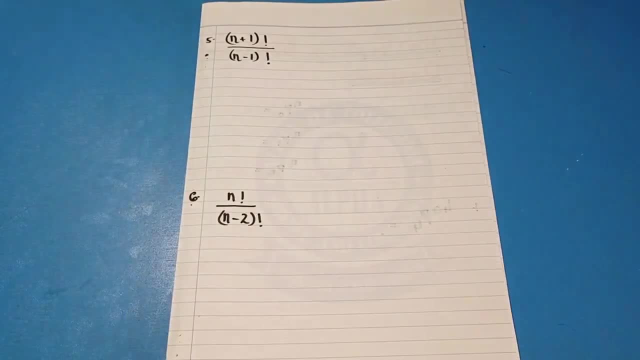 And then your answer will come numerically. Okay, son, Now I have seen two further questions for your convenience, And this is a very important question. The first question is that the variable factorial questions have come. The variable factorial questions are more important to keep in mind. 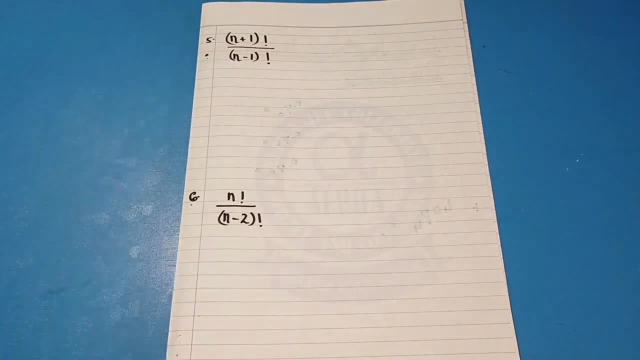 So what is the difference between the number factorial and the number factorial? The number factorial is the number of factorials divided by n-1 factorial. We were doing numerically factorial questions, which means the numbers factorial, And if the number factorial sign is being divided. 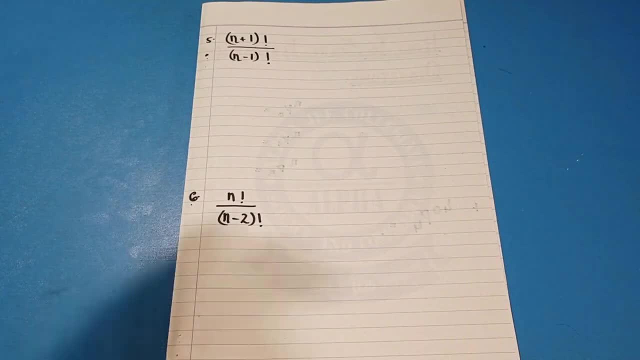 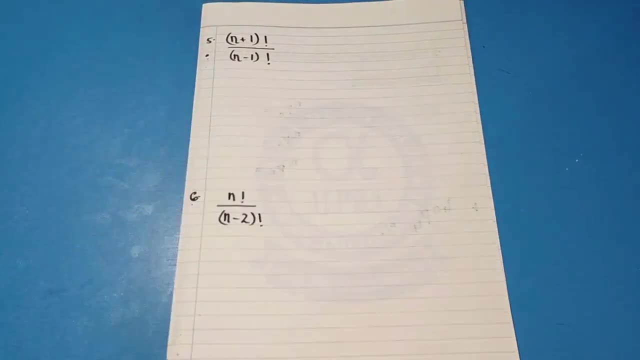 by two factorial, then what would we do? So the concept there will be applied to us here. What does that concept say to us? That you have to expand the big factorial so that you can cancel out the smaller one. So that is the concept, son. 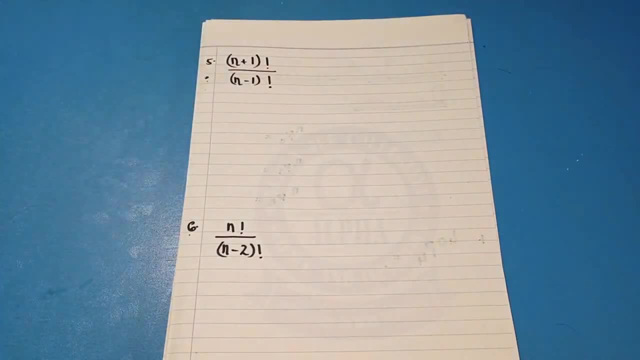 So the concept is n-1 factorial divided by n-1 factorial. My son, what will you do? First of all, you will analyze what is the big value. Is n-1 big or n-1 big? You should know this. 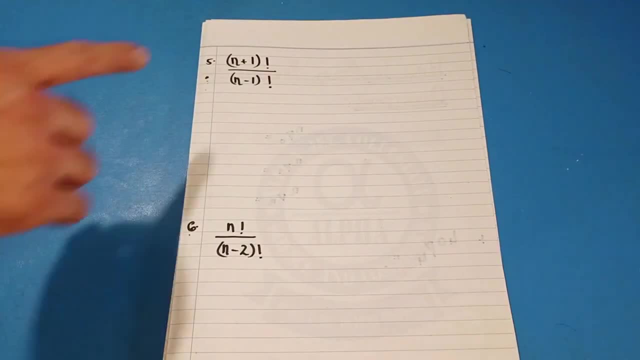 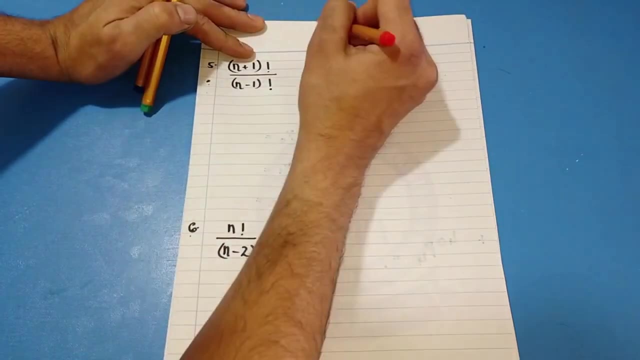 My son, the further you go in minus, the smaller the number becomes. So what is your big value? n-1.. Now, how will it expand? You should know this. Look, we open the factorial sign and it keeps expanding from 5 to all the previous numbers. 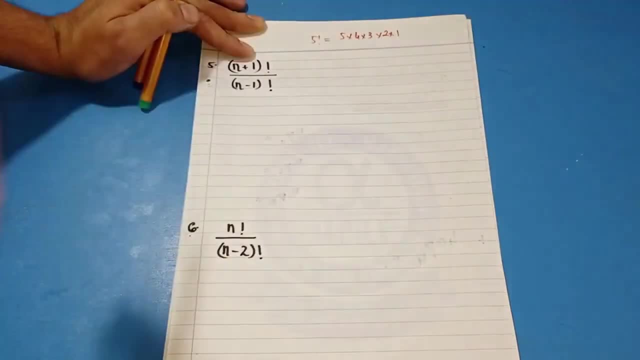 5 x, 4 x, 3 x, 2 x 1, and so on. 5 x, 4 x, 3 x, 2 x 1, and so on. 5 x, 4 x, 3 x, 2 x 1, and so on. 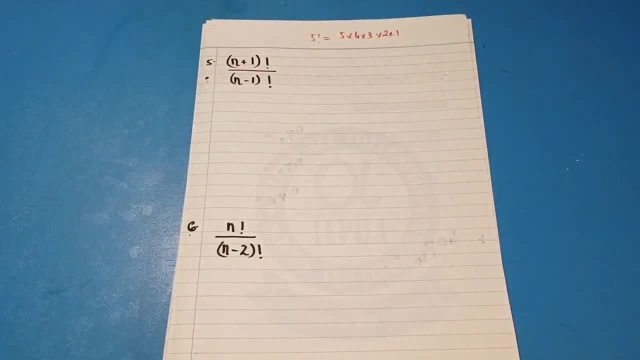 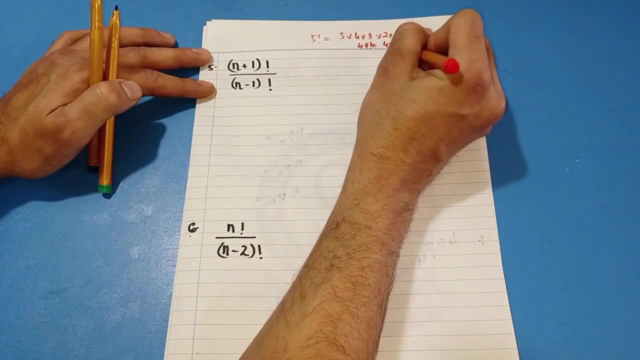 That means whenever we open the factorial sign, it keeps going to the back side. It happens like this, For example, if we take 49 factorial. 49 factorial means 49 x 48 x 47 x 46 x 44 x 43 x 42. 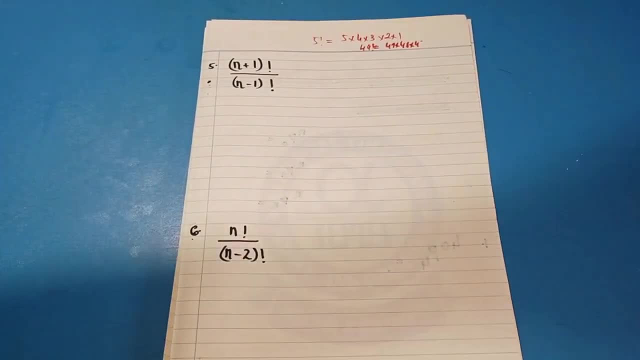 49 x 48 x 47 x 46 x, 44 x 43 x 42, and so on till 1.. Is it clear, son? So what is the property of factorial? When it is multiplied with a number, it will go to the back side. 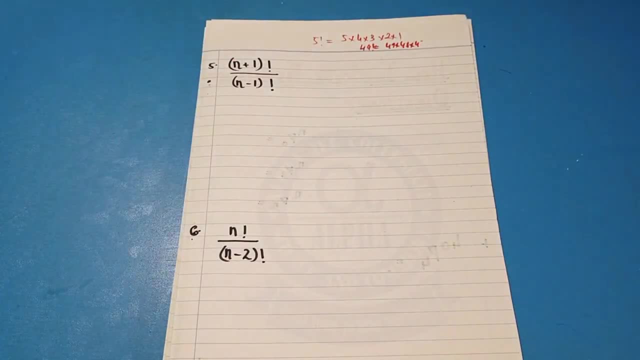 Now, what is coming here? n-1 factorial divided by n-1 factorial And this type of question. blanks are easily available on the Aperture side and Intermediate side. So what is the first thing you will do? You will check which is the big value. 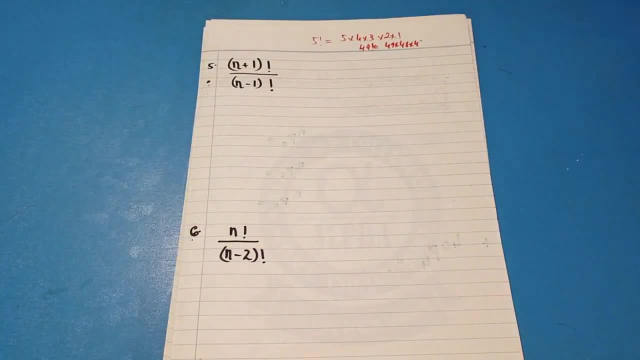 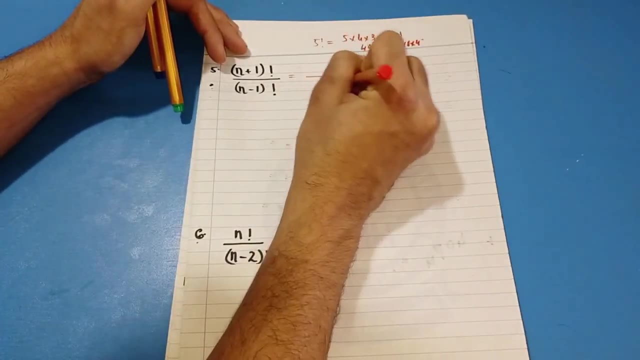 among these. So obviously, n-1 will be big and n-1 will be small. Now you have to see how to open the expand. So, son, how do we open it? Look, you don't have to move the thing below. 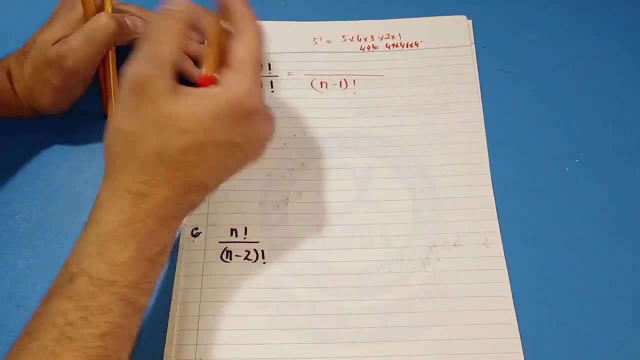 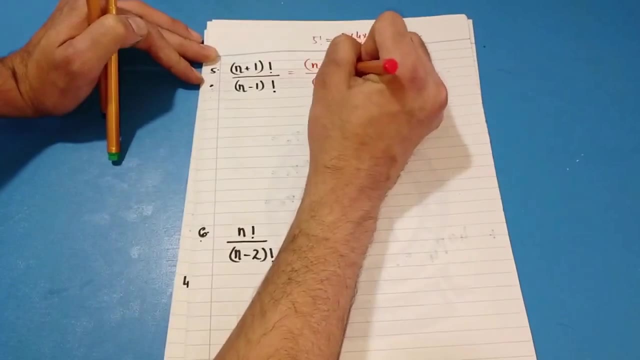 Now look how do we open it. If we open it like this, it goes to the back side. So, son, if n-1 is factorial, then we will write n-1 factorial as it is. Ok, sorry, we will write n-1 as it is. 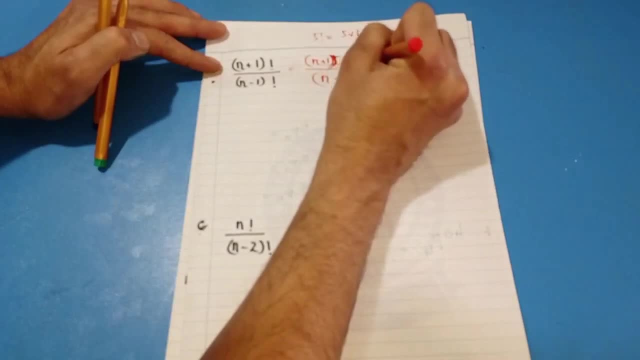 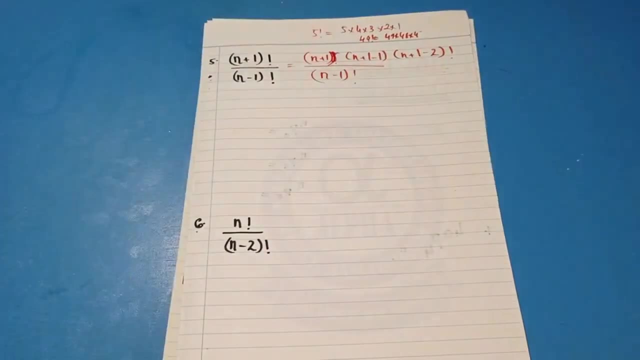 and then we will expand it further. How will we expand it, son? Next time it will be n-1., Then it will be n-2. And we will leave factorial here. What have I done here? Let's see it again. 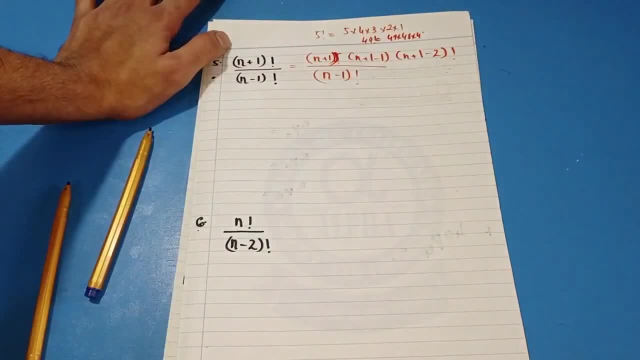 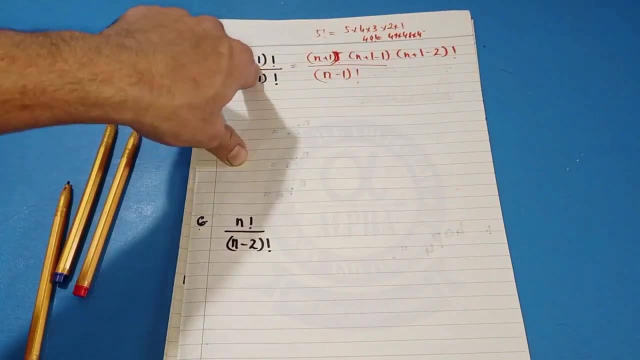 What is the first thing we are doing? We have checked which is the big value among these. We know that it is n-1.. Now we have to expand it. How will we expand it? One number is at the back. So, son, it is n-1.. 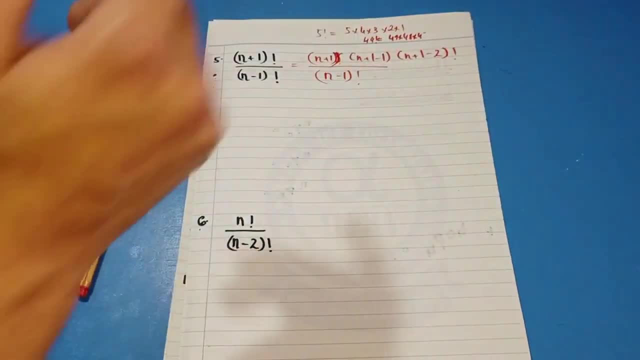 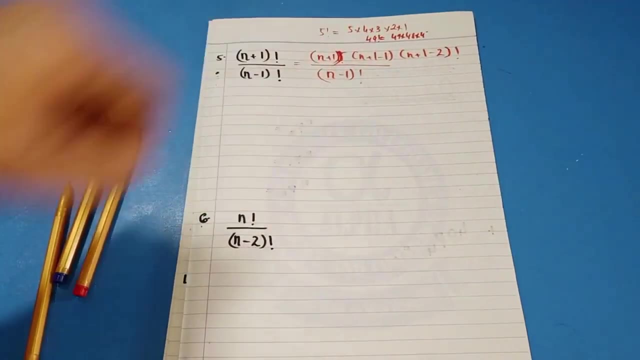 So what will we do? n-1. How do we open factorial? If it is 5 factorial, then we will write another number of 1-1 out of 5.. Then we will write another number of 1-1 out of 5.. 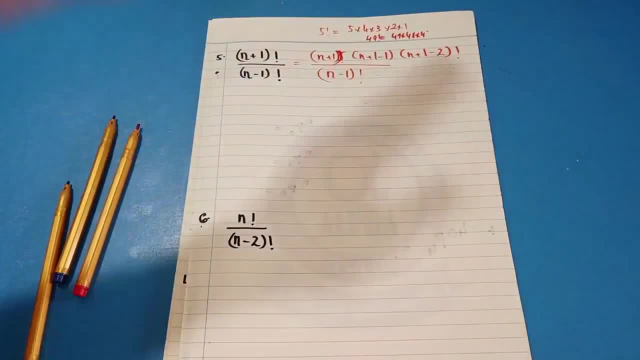 Then we will write another number of 1-1 out of 5.. That is, 5 multiplied by 4, multiplied by 3, multiplied by 2, multiplied by 1.. How do we get this If I have 5 factorial? 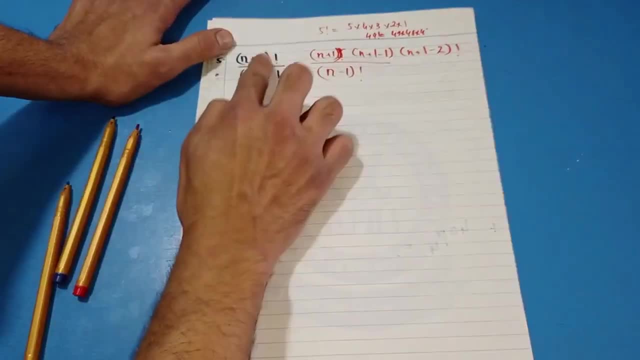 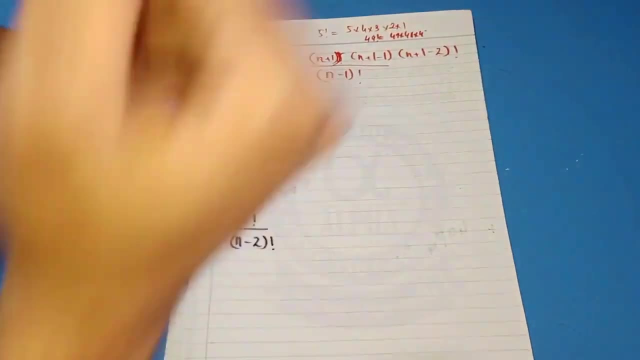 then 1 is 1, so, son, This is the same work being done here. also, son, If n-1 is factorial, then n-1 we write once. then we will multiply 1 from n-1.. Then we will multiply 2 from n-1. 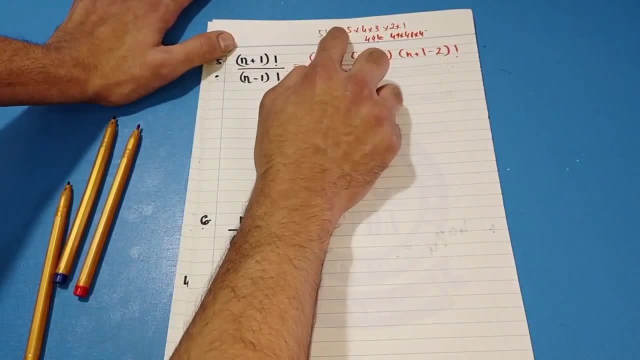 Then we will multiply 3 from n-1.. that means that 5 is 1-4 from n-3,, so 2 from 3, then 2 from 5!. If so, we subtract 2 from 5.. 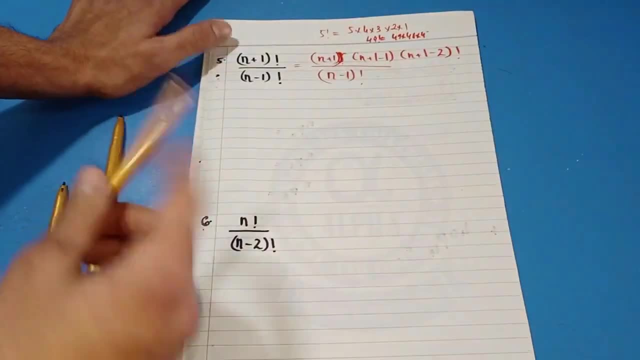 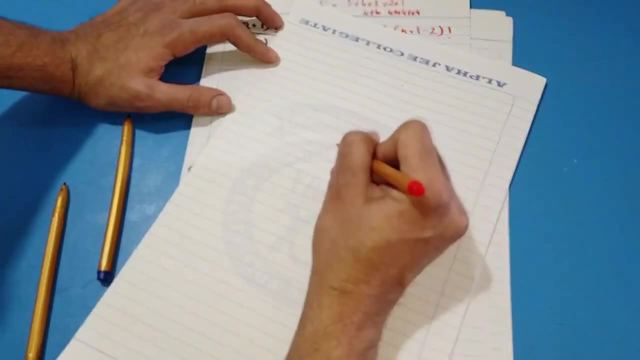 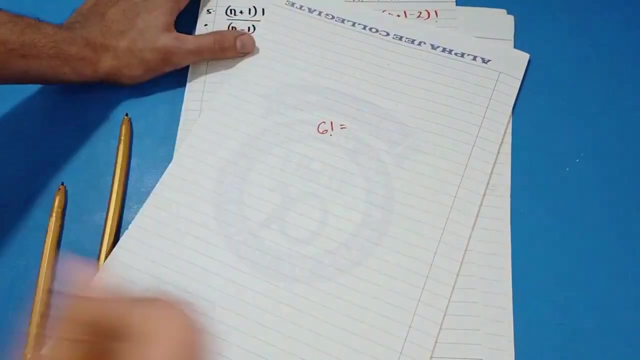 Or if we subtract 4 from 5, then we subtract 1 from 4.. Are you able to understand this, son? By the grace of God, have we clear our ends with so many of these? Now, for example, you have 6 factorial. I know it is difficult for the first time. if you have 6 factorial, then how will you open it? 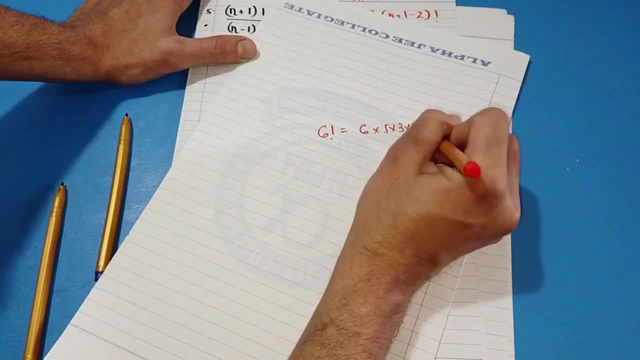 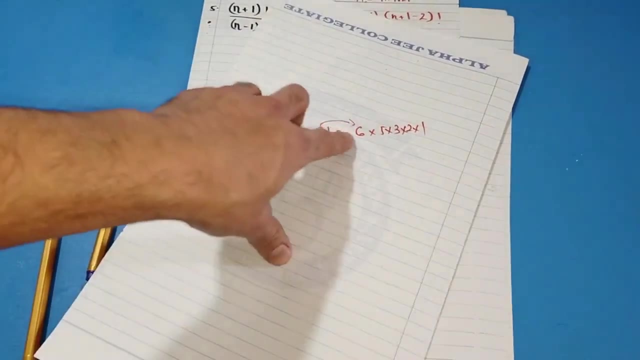 How will you open it? 6 multiply by 5, multiply by 3, multiply by 2, multiply by 1, what does it mean? What exist? an expand factorial, and how will you escape? first, write 6 as it is and minus 1 from 6, it becomes 5. 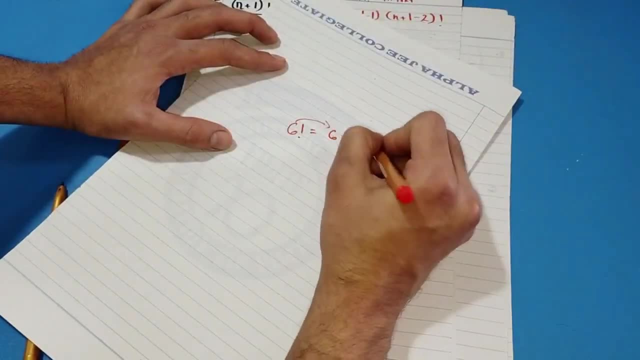 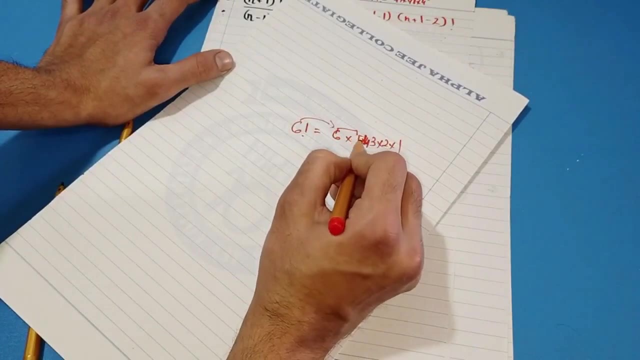 After this, you have minus 1 from 5, so you will have 4 and 3. it be only minus 2. So what is the meaning of this? 1 minus 1 in original term becomes 5, 2 minus 2 is 4 and 3 minus 3 is 3. 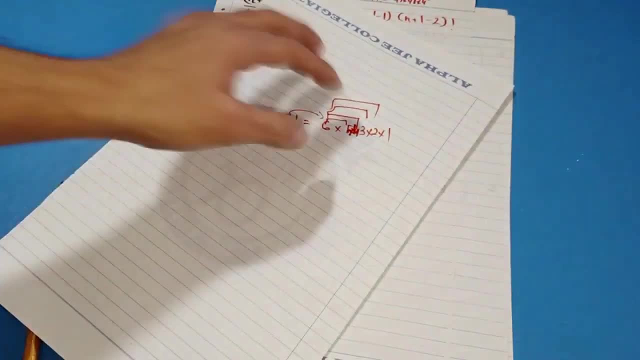 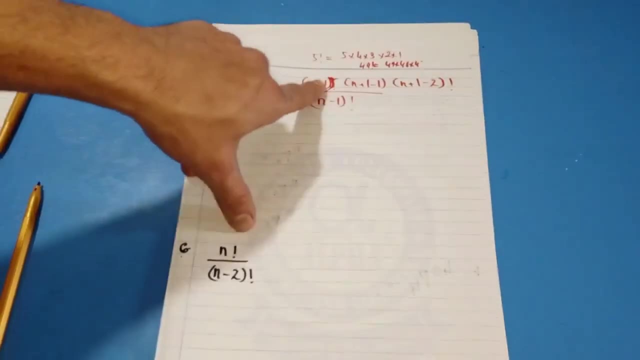 and minus 4 from original term is 2 and minus 5 is 1. We are doing the same thing here too. and what are we doing? If I want to expand this term that it is n plus 1,, then n plus 1 will be written once. 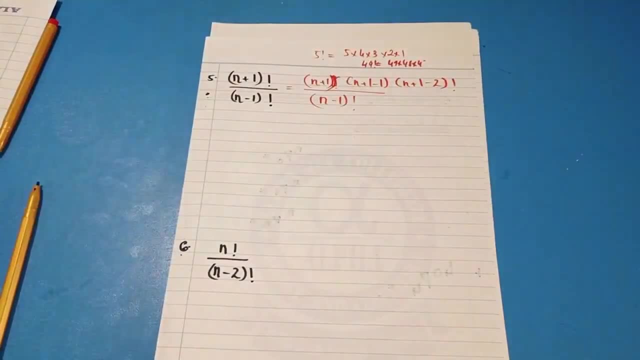 what will happen n plus 1 minus 1, then what will happen n plus 1 minus 2, and I will stop here. I will stop here because what will happen to 1 minus 2? Minus 1, and the upper term will cancel out the lower term. 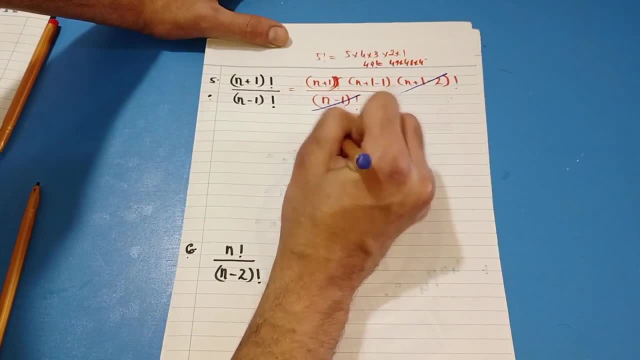 And what will happen? It will be made in a simple way: n plus 1 as it is, and when plus 1 minus 1 is over, then simply n comes. So what will be its final answer? n into n plus 1.. 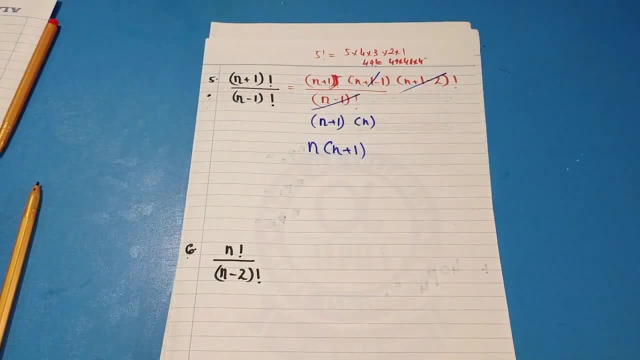 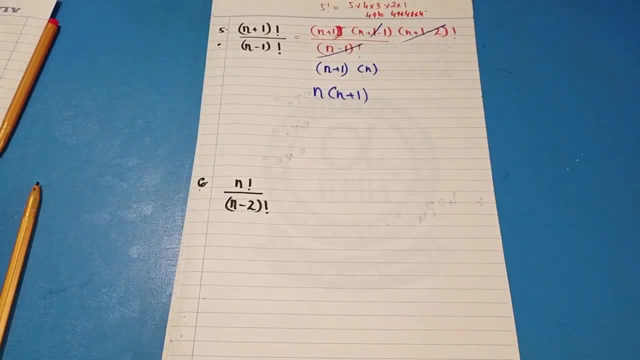 So whenever you get a question- n plus 1 factorial divided by n minus 1 factorial, How will we solve it? My son, we will solve it on this pattern. Now see, I have another question coming. What is coming? n factorial divided by n minus 2 factorial. 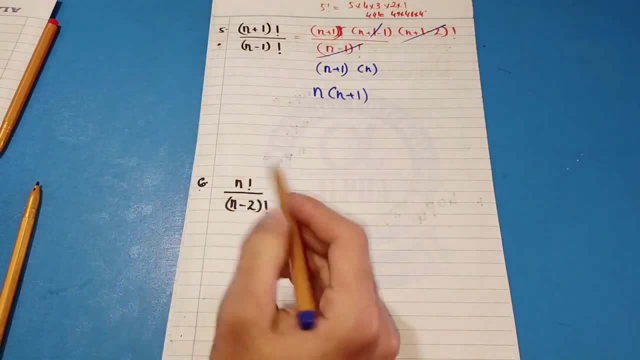 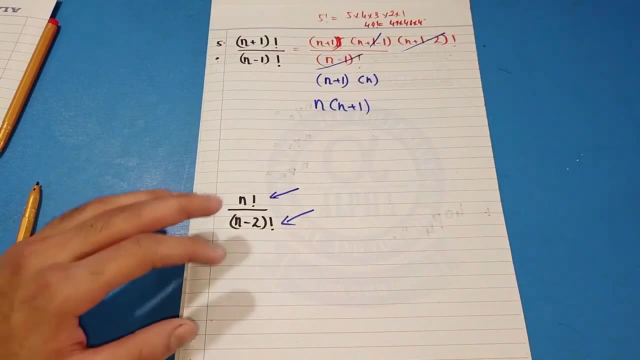 My son. how do we solve such questions? It is a very easy way, Because the first thing to do is to analyze that if two factorials are divided, then which is the big value? You assume which is the big value. It is clear that n factorial is a big value. 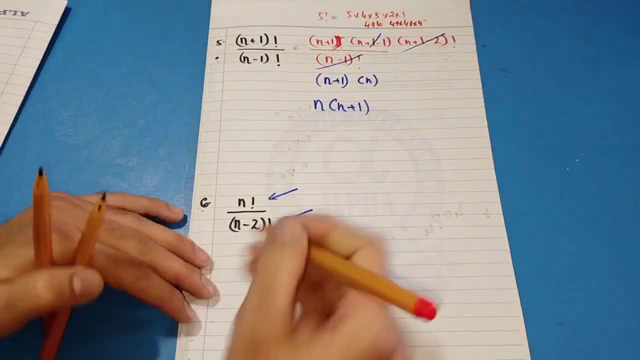 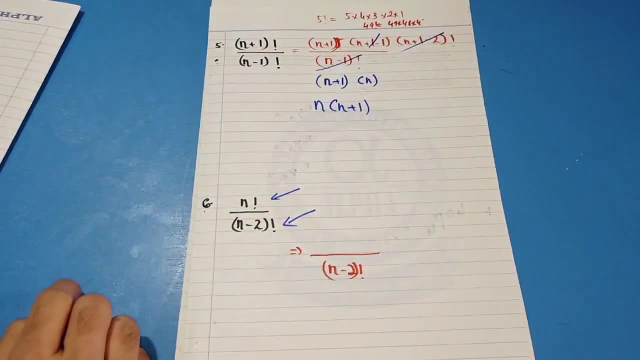 n minus 2 is a small value. Now you have to expand the big value. How to expand it? Let's see My son. the one below will remain n minus 2 factorial as it is Now. if we have to expand n factorial, 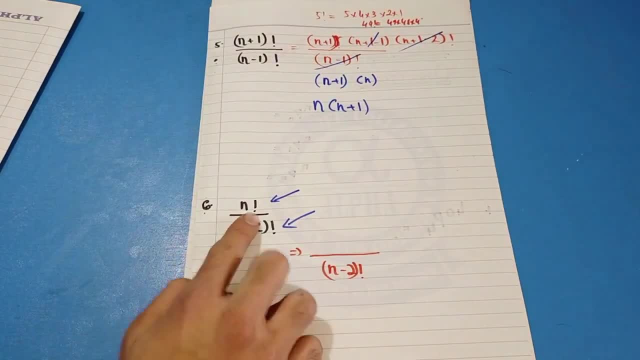 then how will we expand it Here? what is the number n, n factorial? Now we have to expand it, That is, we will do 1,, 2, 3 minus from it. So what will happen? 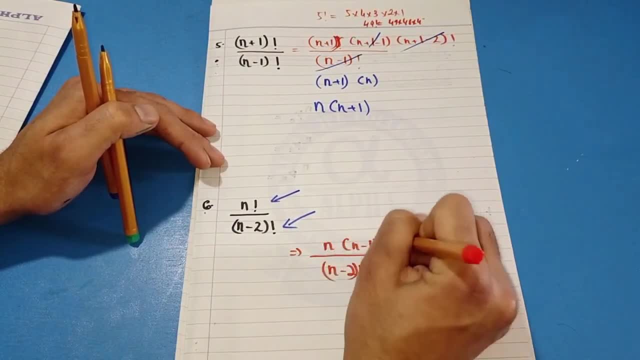 It will happen that n will be written like this for the first time. Then n minus 1 will happen once. Then what will happen? n minus 2.. And here we will stop it by applying factorial sign. How will the n minus 2 factorial from the upper n minus 2 factorial? 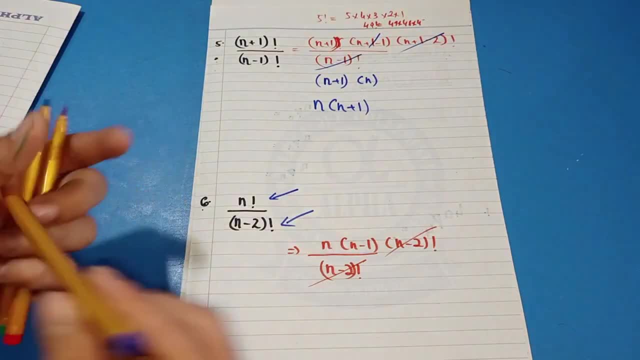 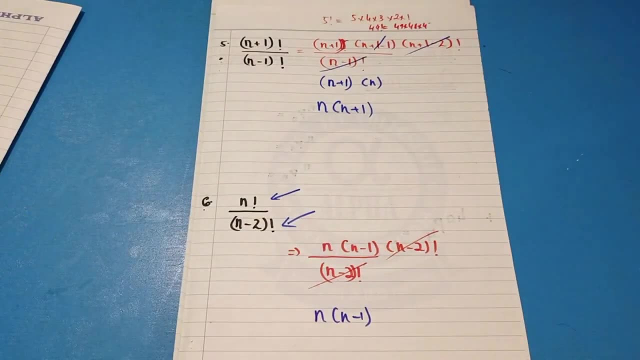 get out from the lower n minus 2 factorial. So what will be the answer to this particular term? What will it be n to n minus 1.. And here we complete a major part. My son understanding the questions of factorials is very important if we want to. 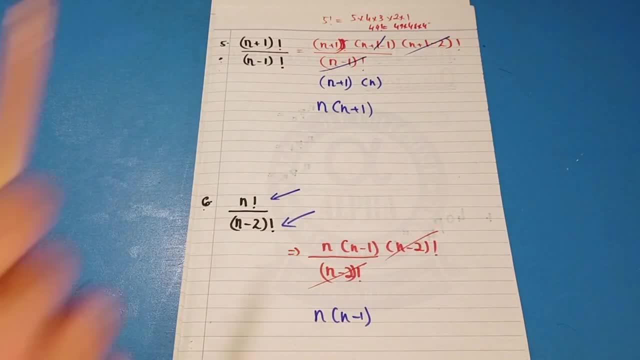 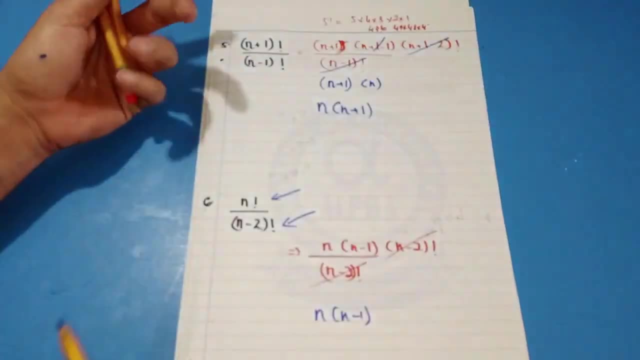 What did we understand? What did we understand in this particular lecture? How to solve factorials. I will repeat these two again if any of you have any issue. The first thing, whether it is a numeric value or a simple variable in the form of factorial location, 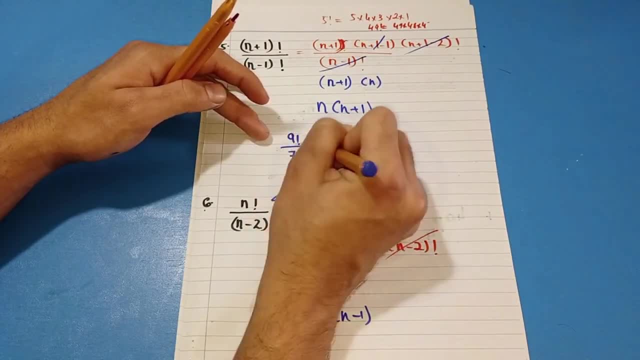 Your first task. for example, if 9 factorial divided by 7 factorial comes, What you have to do first is to check which is the big value among them. The answer is clear: 9 factorial divided by 7 factorial. What you have to do first is to check which is the big value among them. 9 factorial divided by 7 factorial. What you have to do first is to check which is the big value among them: 9 factorial divided by 7 factorial. What you have to do first is to check which is the big value among them. 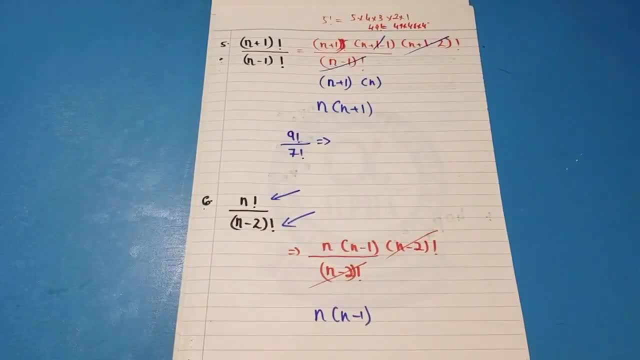 So what you will do is expand 9 factorial. How far will you expand Up to the bottom term and then after that you will put the factorial sign so that the term from the top cancels out and your simple numeric form gets data. 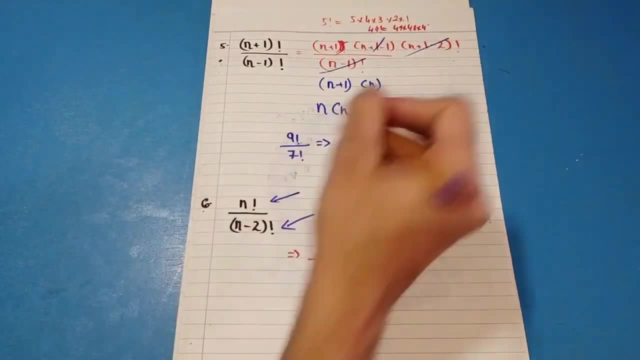 So what will happen? How far will I expand 9 factorial? Obviously, on the top is 9 and at the bottom is 7.. So what will I do? 9 into 8, into 7.. I will stop here. 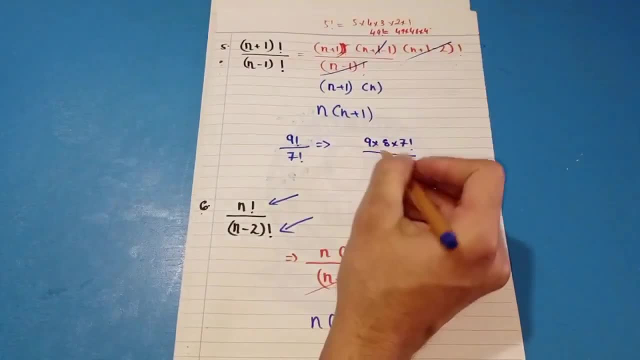 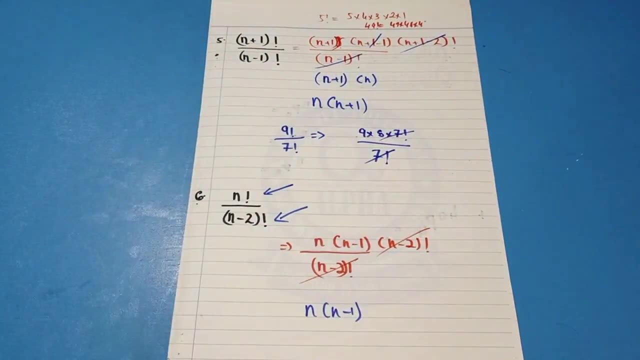 After stopping I will put the factorial sign so that I can issue property further And from the bottom of 7 factorials, 7 factorial is finished. So what is left? 9 into 8.. and how to do variable one is very easy. 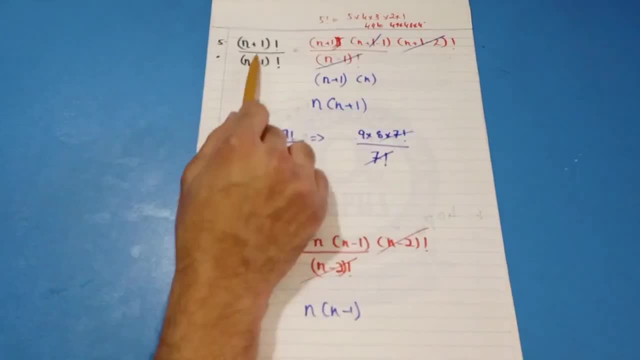 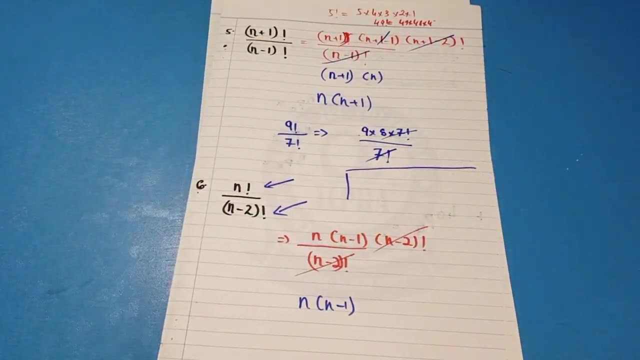 the easiest way to do it is to analyze. for example, if you are getting this question, what will you do first? you will analyze how to analyze which is the big term. it is clearly written: n plus one factorial is big term and n minus one factorial is small. 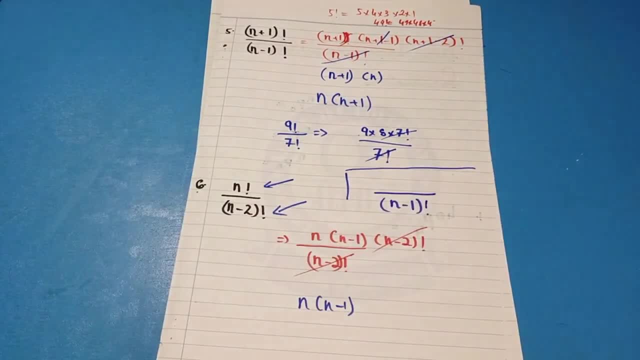 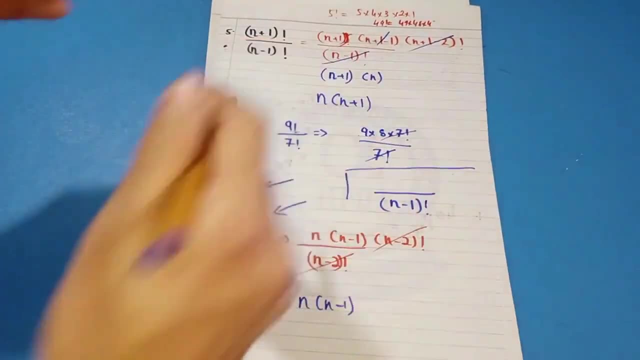 so you will give the small one the address and you have to do the work of big one. how to do the work? you have to open it and expand it. how to expand? if you understand the numeric term, then you will understand the variable term as well. 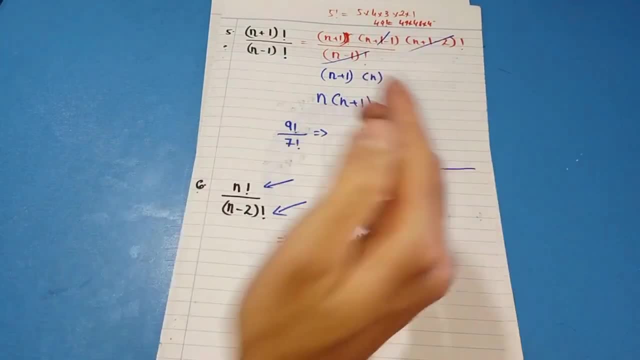 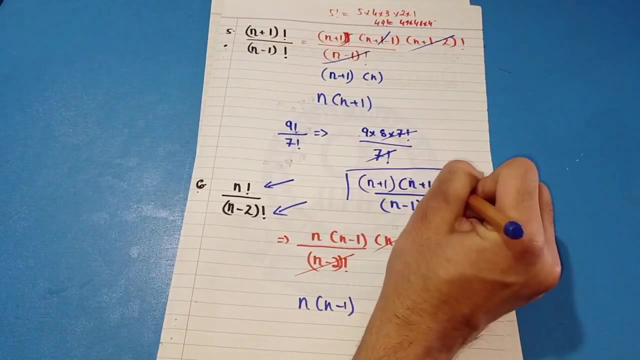 that once you will write that term as it is and then every time you will do one minus from that term. now what happened? the first time it was n plus one. the second time it will be n plus one minus one. then what will happen? one more time you will do one minus from the original term. 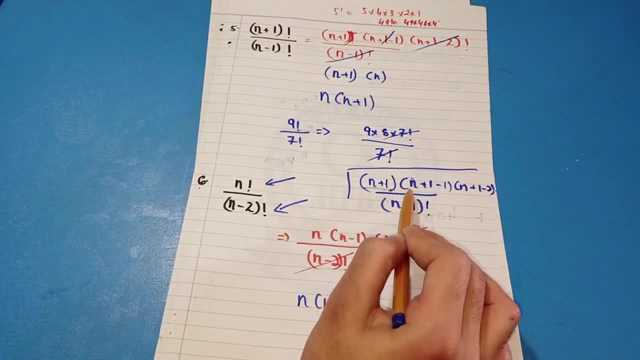 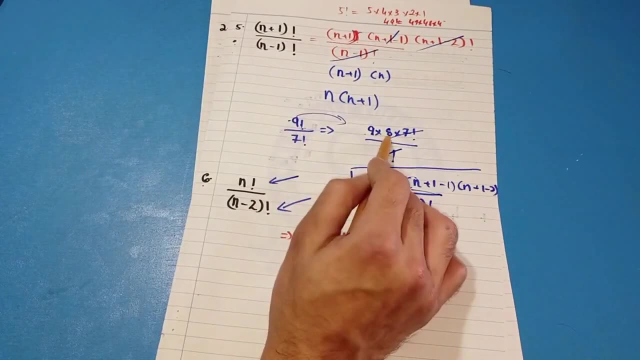 then what will happen? n plus one minus two. that means you have to write the original term once and do one minus from it, which we were doing in the simple numeric term. once you do one minus from the original term, then once you do two minus from it. 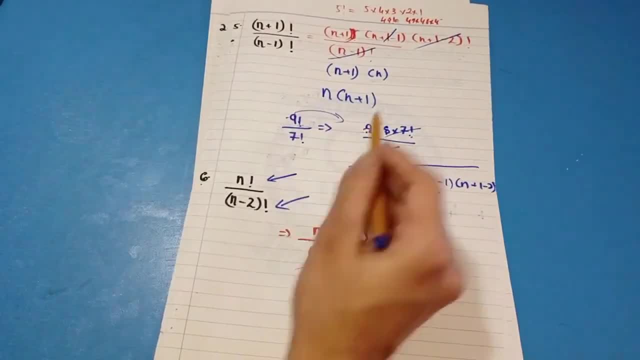 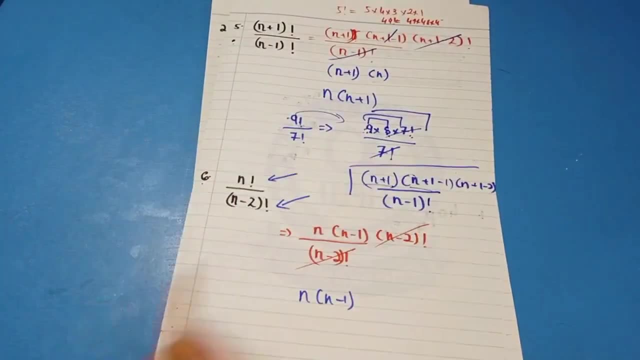 what is this? 9x8x7x6x5x4x3x2x1. this is the thing that if you write the original term once, then if you do one minus from the original term, then it will be 8. if you do two minus, then it will be 7. 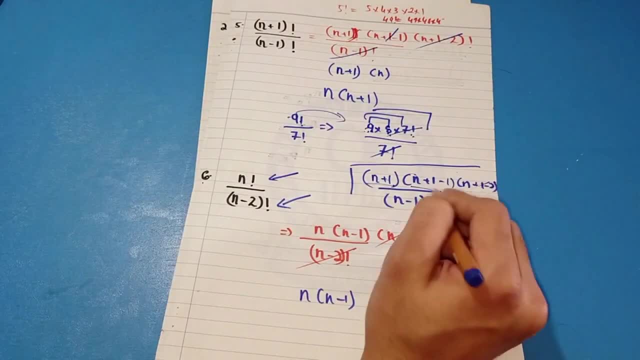 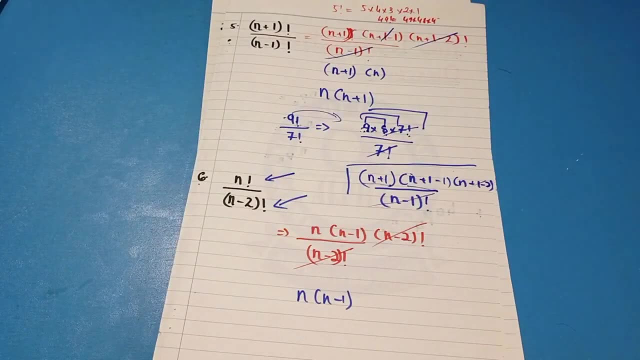 if you do three minus, then it will be 6. if you do more minus, then it will keep on going. so this concept is for the same variable. if you are able to understand my question, then i guess you will understand it. that's why i made a separate lecture video on it. 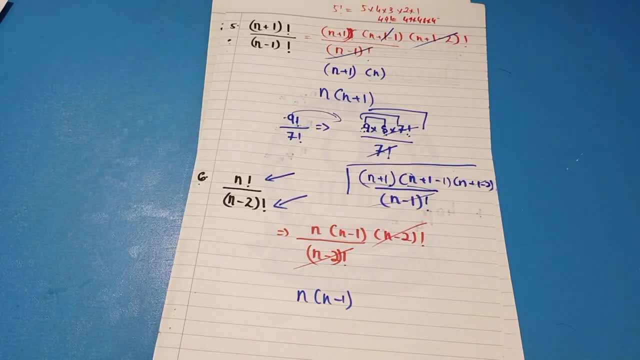 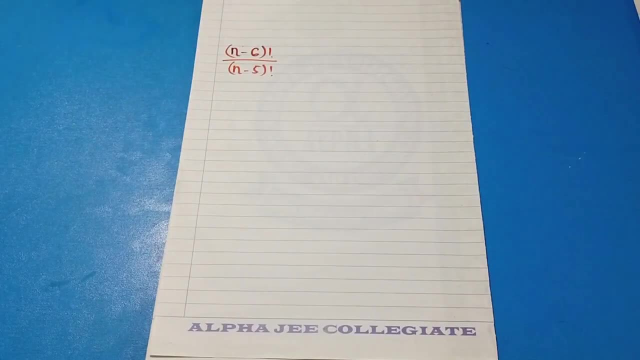 so that you can learn some basic ways of doing intermediate values. it is important to learn these things without any hesitation. factorial concept is an important concept, without any hesitation. ok, son, now, at the end of this lecture, i want to give you one more concept. for example, we got a question like this in the paper or in mcqs: 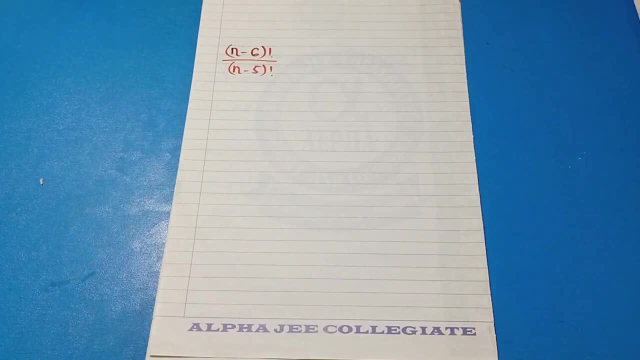 what is it saying? n minus six factorial divided by n minus five factorial. how will you solve it? see my son now, both these terms are coming in minus. what did i tell you? you have to analyze the first thing first, that what is the big value? see, n minus six is also big, or n minus five is big. 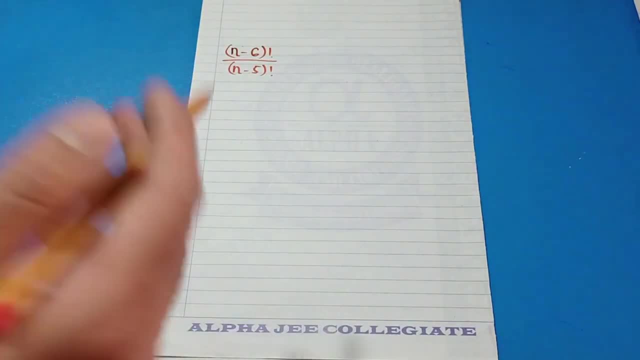 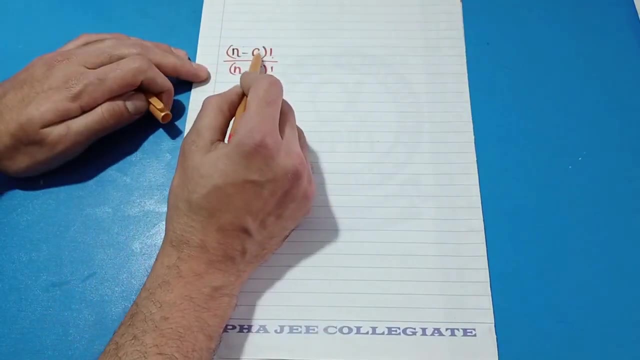 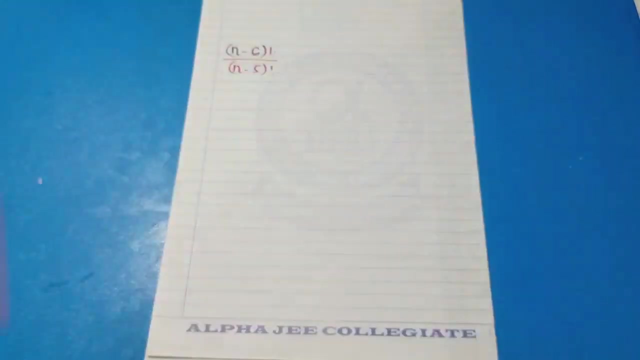 you should know this thing. see in minus: as you go ahead, your number keeps getting smaller. so you should know these basic things. now see what is happening: n minus six factorial is being divided by n minus five factorial. now, if you want to solve this, then you will expand that part, which will be big. 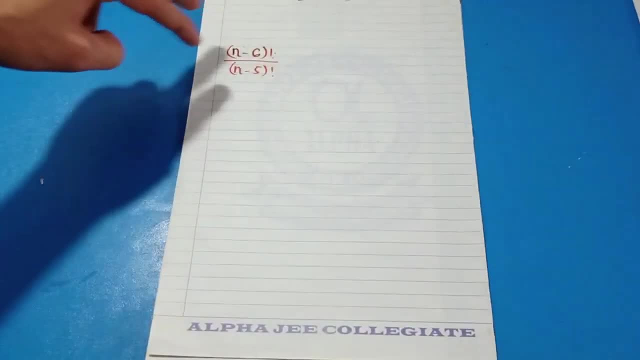 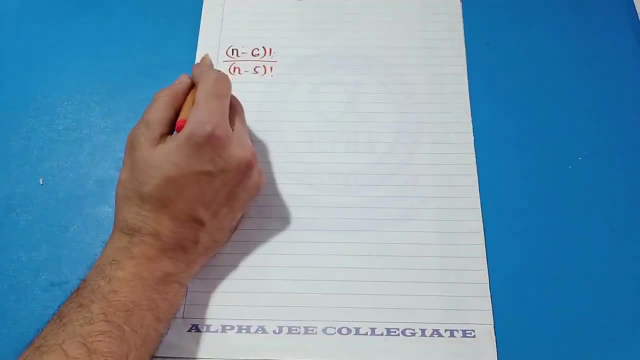 or you will expand that part which will be big. now, first of all, we should know what is the big value between these two: n minus six is big or n minus five is big. now the majority of people's concept is so bad that they say that, sir n minus six factorial is big. 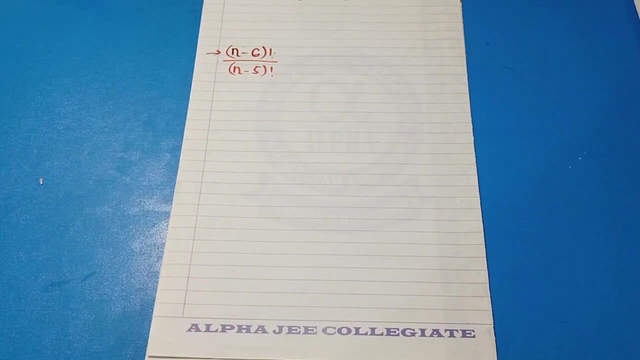 now in minus. as you go ahead, your number keeps getting smaller. that means n minus nine is a very small number as compared to n minus six, or if i take minus twelve or minus fifteen or minus hundred. all these numbers are very small as compared to zero or one. 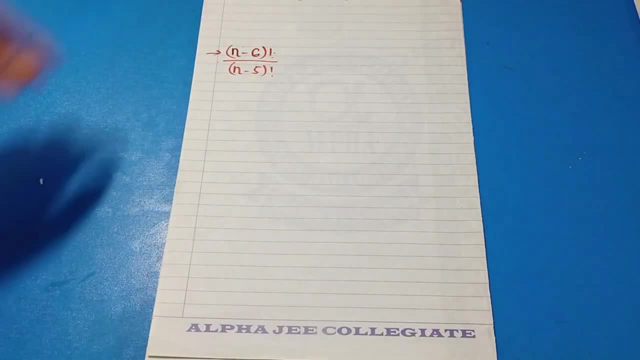 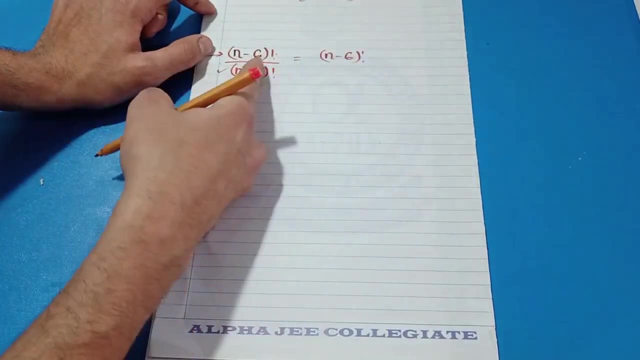 as we go ahead in minus, our number keeps getting smaller. so which is the big number? so how will we expand it? this question comes without any hesitation. so what is the small number? n minus six factorial: it will remain as it is on its place. n minus five factorial is the big number. 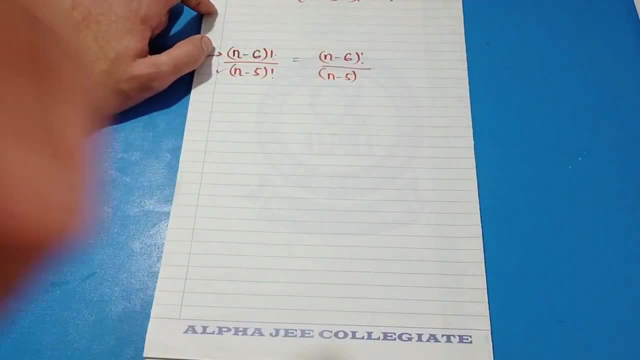 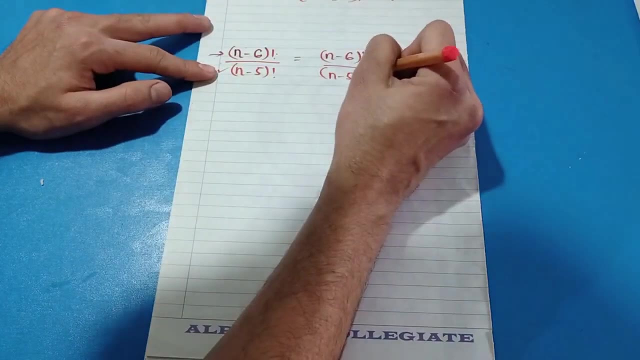 how will we open it in the first time? n minus five will remain as it is. then we will minus one number from n minus five, which we were seeing in factorial question, that you have to write the original term once and then you have to minus one from the original. 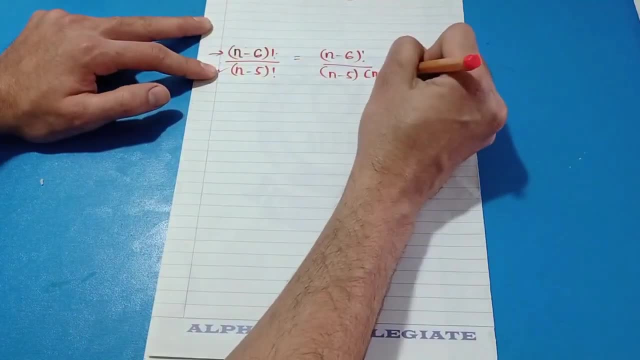 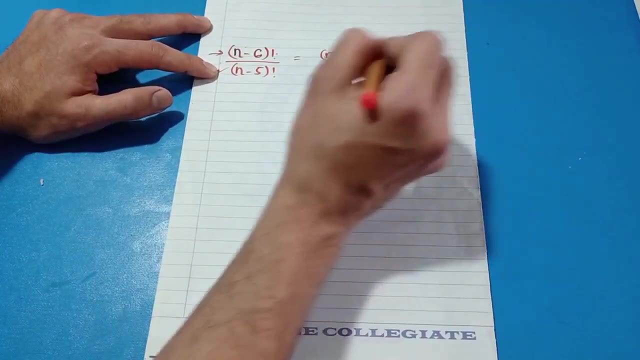 so what will become from n minus five when i will close minus? so what will become minus six? what did i say when i will do minus one from n minus five? so what will become minus six? that is why we will not expand it by putting factorial here. 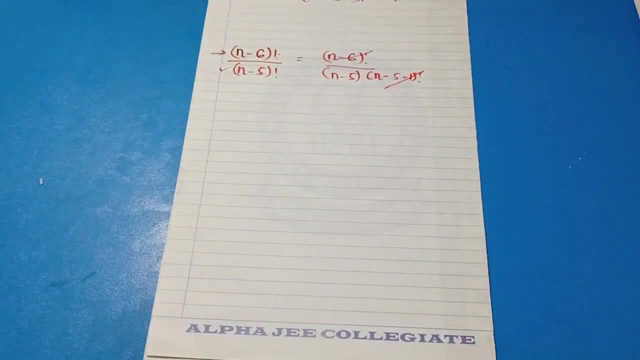 we will stop it here, because n minus six factorial below n minus six factorial, how will it be allowed? and directly, we will get the answer: one divided by n minus five. what will come, son? one divided by n minus five. is it clear to you? i guess, inshallah, this thing will be clear to all of you. 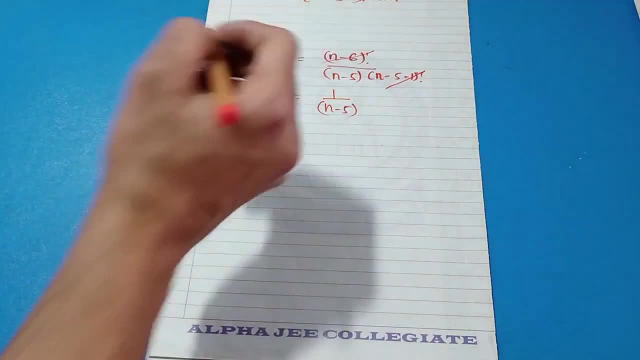 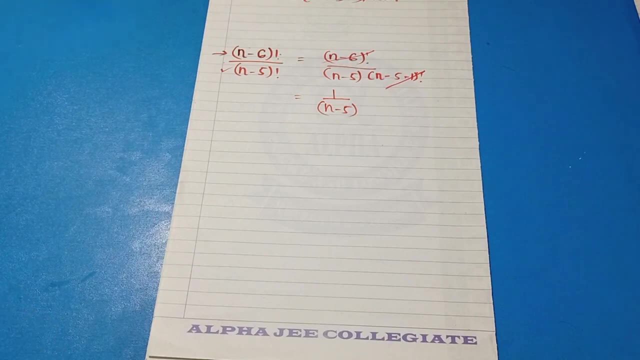 what did i say? i will repeat it again quickly, in a simple way. whenever you have two terms- factorial, based on minus- how will you solve it? first of all, you will analyze it. the same old thing that: what is the big value, what is the big term from these nine? 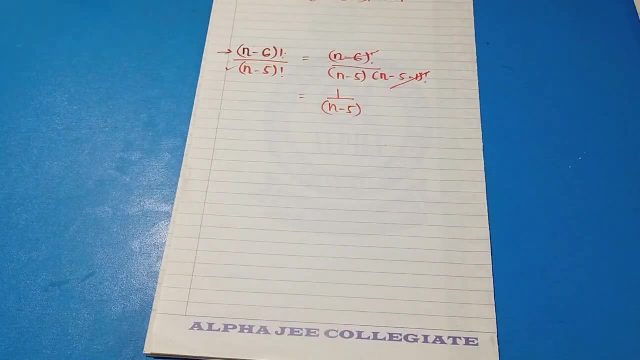 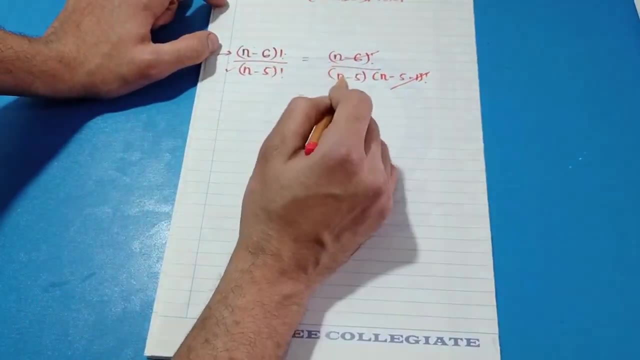 it is clear that the big one in minus is basically a small number. so n minus six is a small number. so n minus five factorial is big. we will expand it. how will we open it? we will let the original term be edited once. then we will do one minus from it. 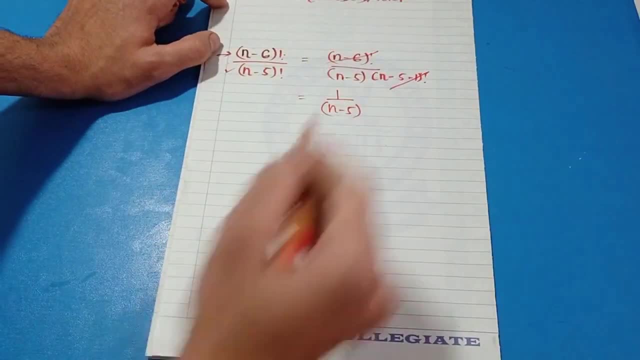 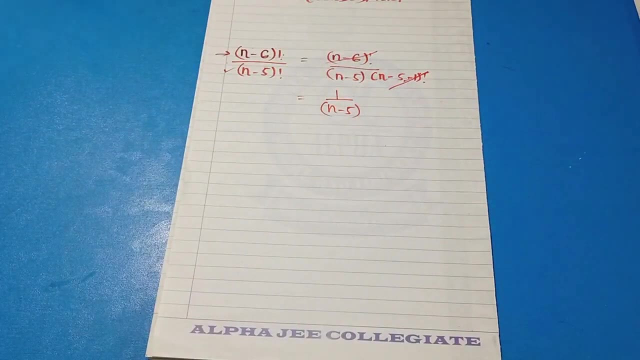 so original is n minus five. if i will do one minus from n minus five, then what will become? n minus six. so n minus six factorial will be cancelled from n minus one. the answer will come in a simple way: it will become my one over n minus five. 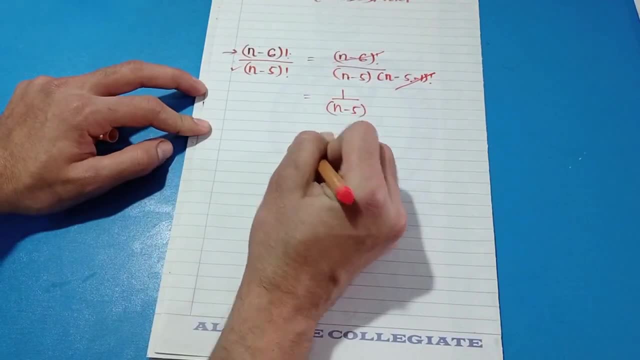 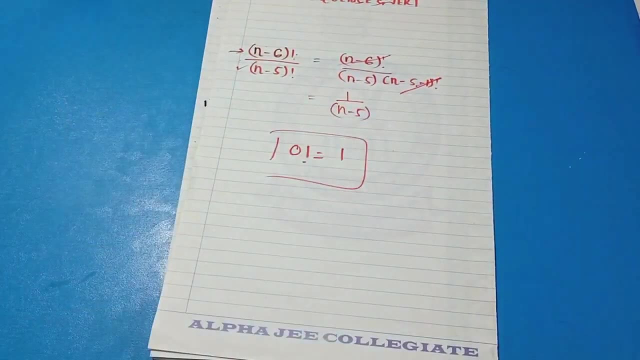 in the last. i want to tell you one more thing. what is zero factorial, my son? whenever the examiner asks you about the value of zero factorial. so what is zero factorial? we have one. what is, my son? the answer to zero factorial is always one. so if i will say one last thing to you, 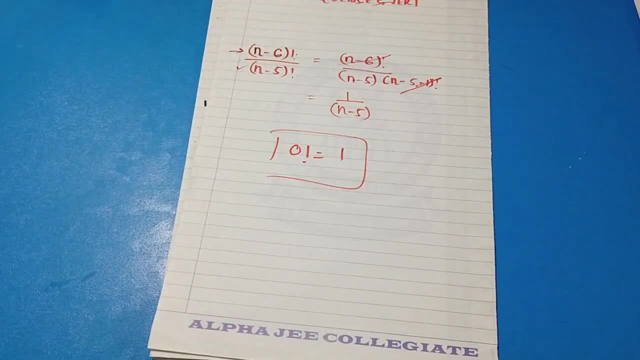 that what we have read in today's video lecture- how to solve factorial but still some topics- are in the book of sin board. i have to go in detail because i know these are very important topics. not only it can take advantage of intermediate, but also it can take advantage of aptitude. 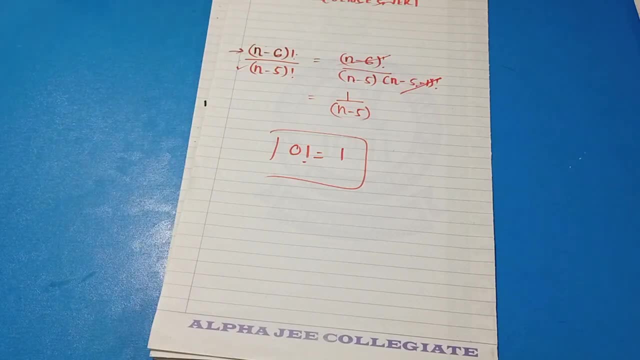 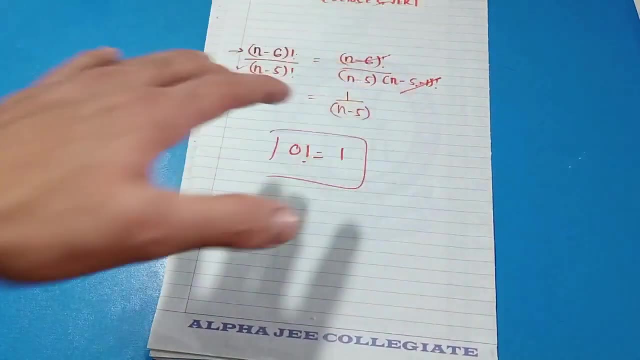 that's why, on the topic of factorial, i have made this video of twenty to thirty minutes so that you can get an idea, not only on the topic of factorial, but also on the topic of the paper of intermediate math. its MCQs have a lot of questions. 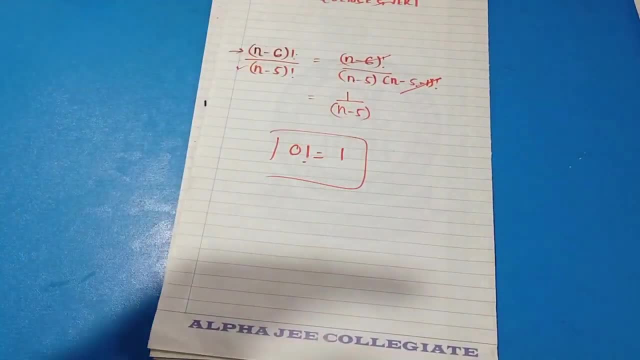 these are the variable ones, but also in the exam of aptitude, whether you are appearing for NAD, whether you are appearing on IB side, whether you are appearing on NET side or you can look up any book of SET. in that you have these factorial based questions.